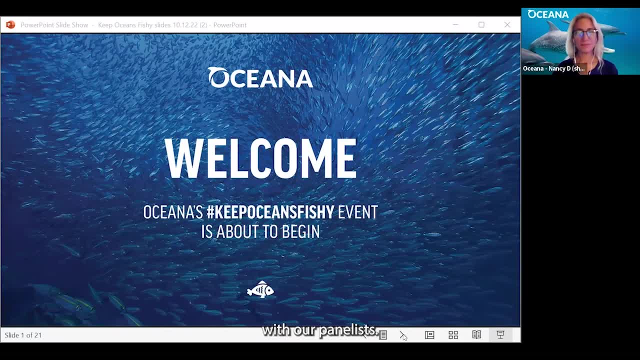 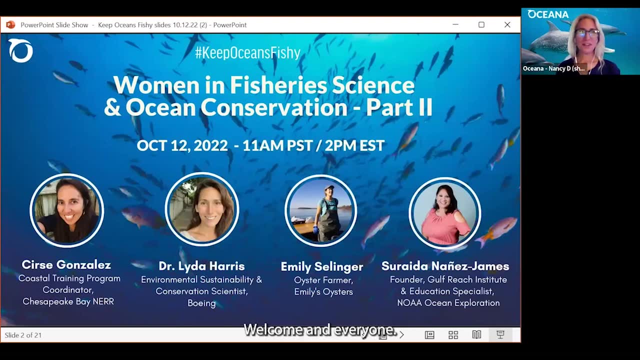 Well, let's get started. Welcome and everyone. thank you so much for joining Women in Fisheries, Science and Ocean Conservation- Part 2.. OCN hosted our first event of Women in Fisheries and Science and Ocean Conservation in September of 2021.. It was so well received. 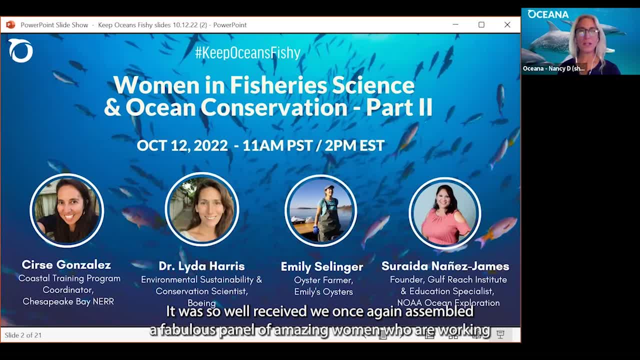 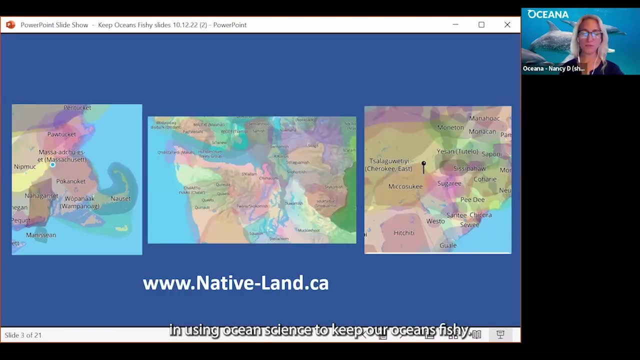 We've once again assembled a fabulous panel of amazing women who are working to protect and conserve ocean resources through science policy, business, education and advocacy, inspiring the next generation of young people interested in using ocean science to keep our oceans fishy. 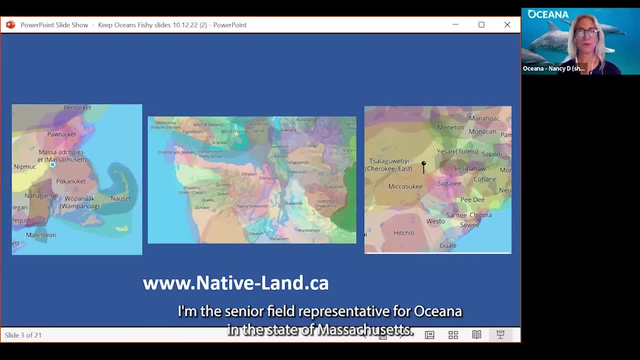 My name is Nancy Downs. I'm the Senior Field Representative for Oceana in the state of Massachusetts. I'd like to begin the program by acknowledging the original peoples and stewards of the land that I'm Zooming in from Today. I'm joining you from Millis, Massachusetts. 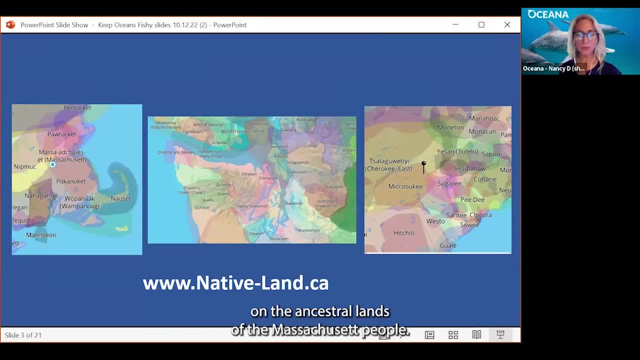 I'm the Senior Field Representative for Oceana in the state of Massachusetts, on the ancestral lands of the Massachusett people. I'm fortunate to be able to do this work on lands that have been cared for by many Indigenous communities of the past, present and future, and today I'm joined by two of my associates in other parts of the country, so I'd like to pass the mic over to Sarah, who will introduce herself. 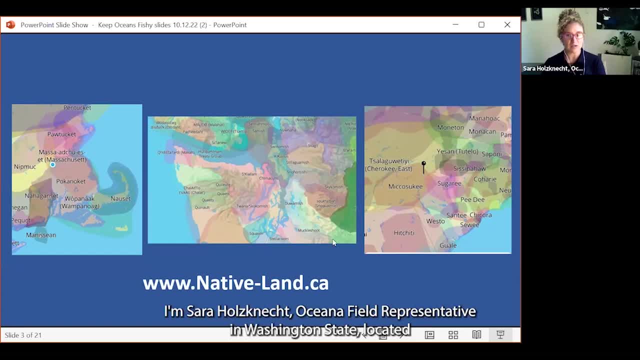 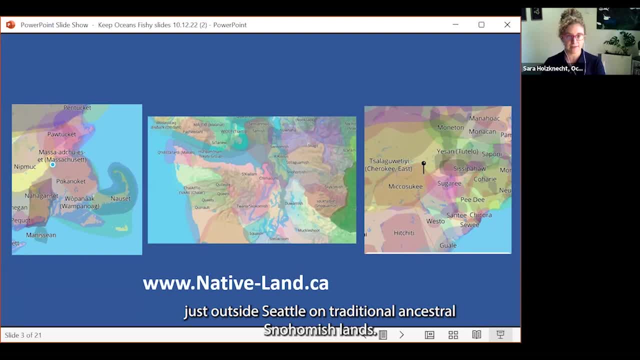 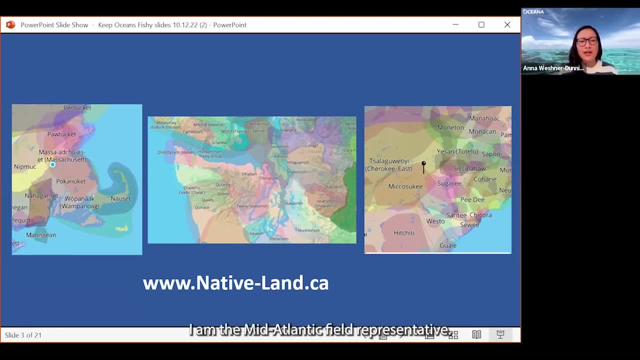 Hi everyone, and thank you for joining. My name is Anna Weschner-Dunning and I am the Mid-Atlantic Field Representative, so working in Maryland and Delaware, and I am currently on Cherokee land. Thanks, ladies, And for those of you Zooming in from other parts of the country, we invite you to explore the history and deepen your knowledge of the Indigenous communities in your local area. 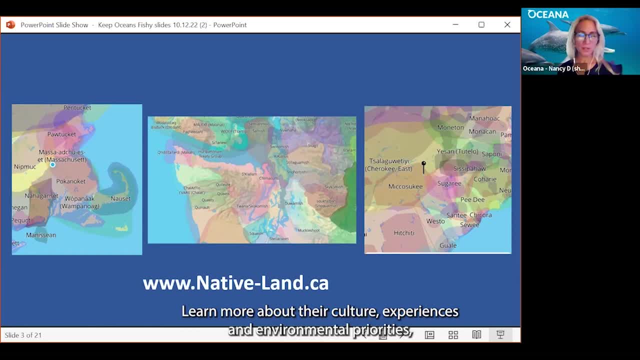 learn more about their culture, experiences and environmental priorities, and do your best to support policies that integrate those conservation principles. One of my associates will be sharing a link in the chat where you can do so. to learn more, And before we hear from our 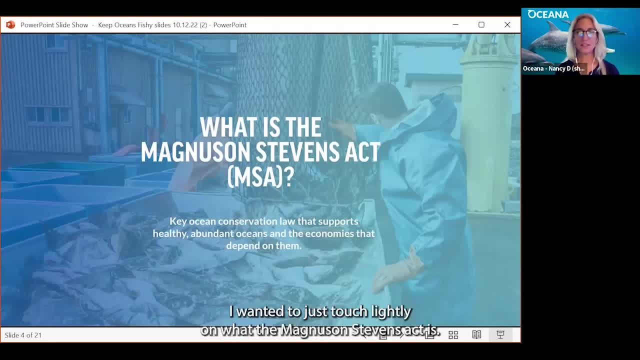 panelists. I wanted to just touch lightly on what the Magnuson-Stevens Act is. This is why we're talking to you today about keeping our oceans fisheries. The Magnuson-Steven Act, or you may hear it called MSA, is our nation's blue ribbon, science-based fisheries management law. It's often 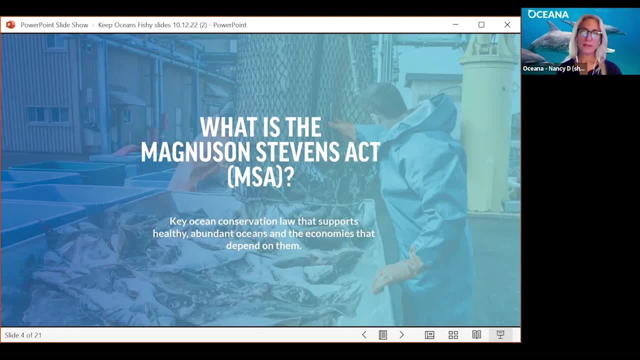 described as the world's envy in fisheries management. The MSA sets the standards and parameters of how we govern marine fisheries in the United States federal waters and fosters the long-term biological and economic sustainability of marine fisheries. Under the MSA, US fisheries 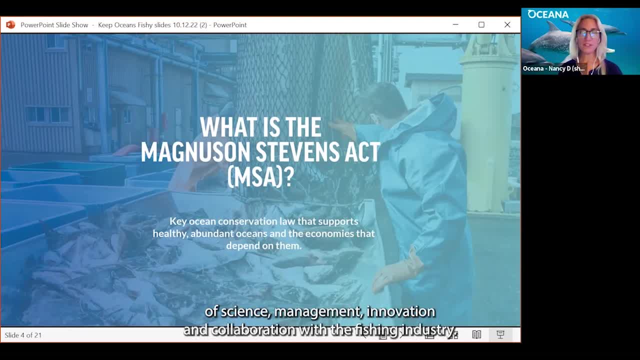 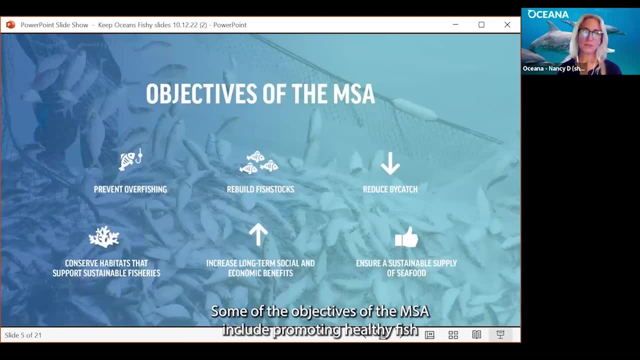 management aims to be transparent and a public process of science, management, innovation and collaboration with the fishing industry. Some of the objectives of the MSA include promoting healthy fish habitat, reducing fishery bycatch, rebuilding fish stocks, improving accountability and representation in fishery management, enhancing fisheries data. 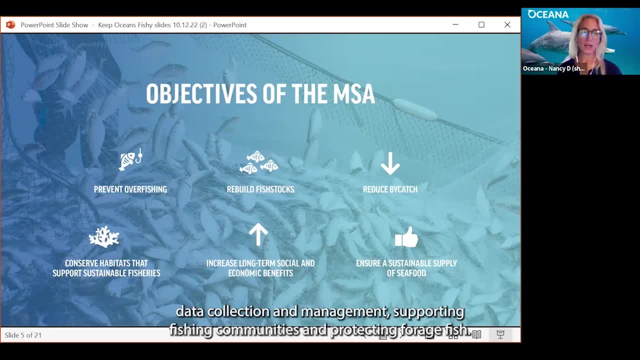 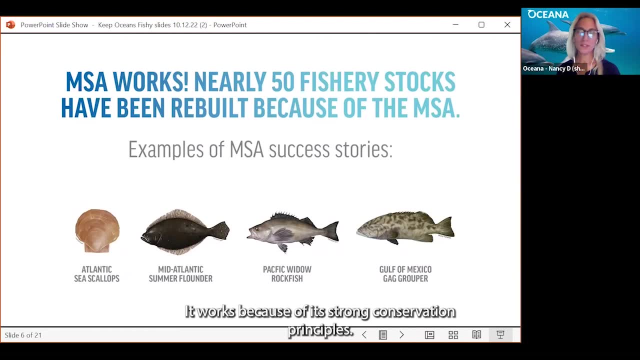 collection and management, supporting fishing communities and protecting forage fish. And I'll tell you what the MSA works. It works because of its strong conservation principles. These are the principles that we're working on. We're working on the MSA, we're working on the. 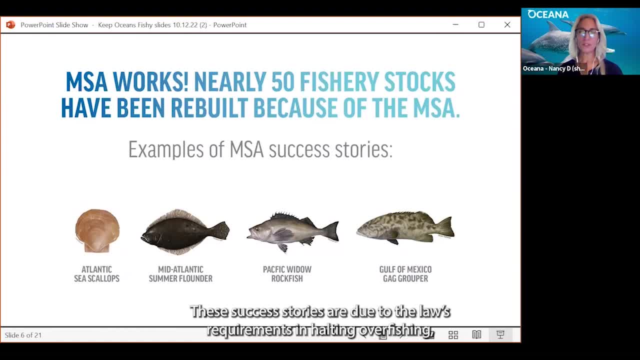 MSA. we're working on the MSA. These success stories are due to the law's requirements in halting overfishing, rebuilding fish stocks and protecting our ocean resources. Thanks to past bipartisan reauthorization of the law, many of our fisheries have come back from the excuse me. 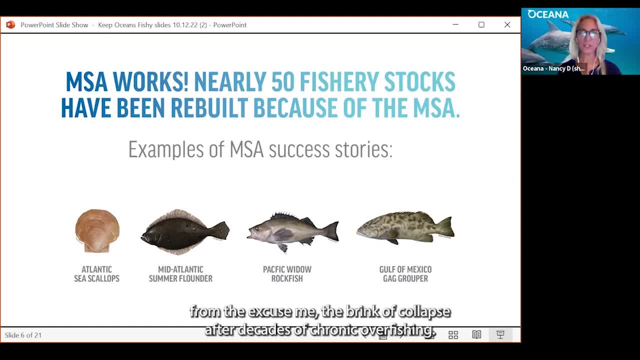 the brink of collapse after decades of chronic overfishing. So thanks for giving me a few minutes to highlight the Magnuson-Stevens Act And now, without further ado, I'd like to pass my mic over to Sarah, who is the Director of the MSA. Thank you, 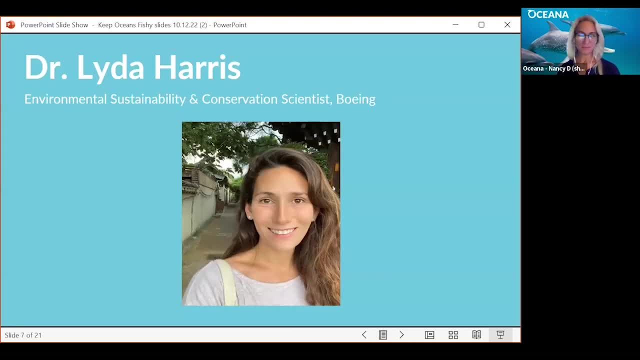 Thank you, Nancy. I'd now like to introduce Dr Lyda Harris, who has recently started a new position as an environmental sustainability and conservation scientist at Boeing. Previously, she was the Clean Seas Research Scientist Lead at the Seattle Aquarium And in this role she managed, led and grew the organization's marine debris program through expanding research funding and partnerships, as well as waste management and. 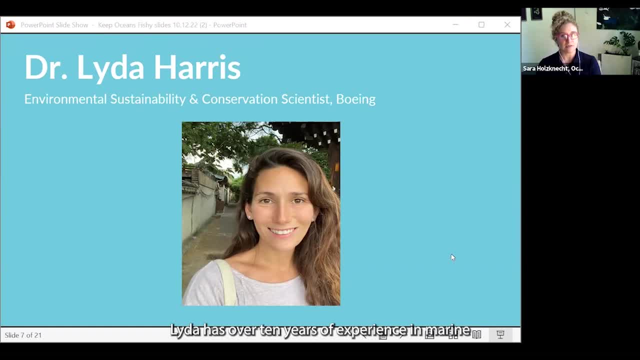 waste reduction efforts in-house. Lyda has over 10 years of experience in marine pollution, data science, zero waste and public policy. She earned her PhD from the University of Washington in the Department of Biology, studying marine microplastic pollution and how it affects organisms, ecosystems and policy. Welcome Lyda. 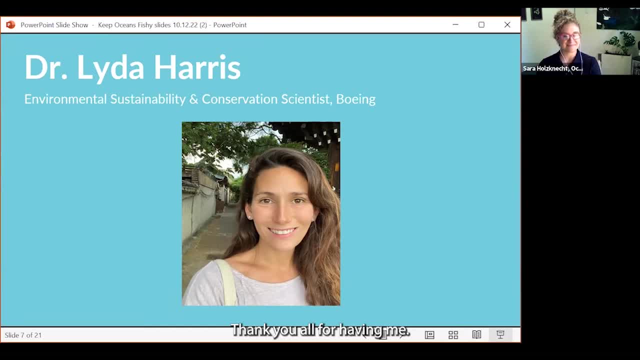 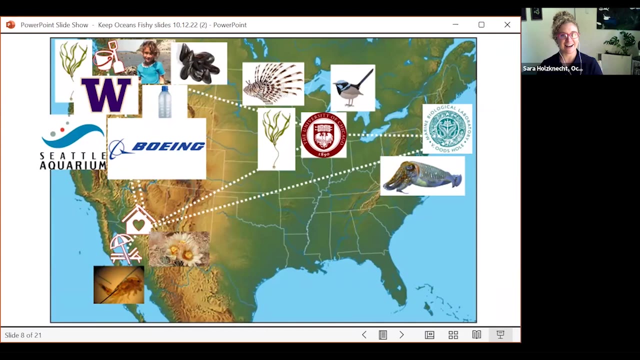 Thank you all for having me. We're so thrilled that you can be here, And can we move on to the next slide please? I think we have a bit more about Lyda's journey. So, as I sort of already mentioned, you've worked across many areas of marine science, as well as geographic regions. Can you tell us a bit more about your background? 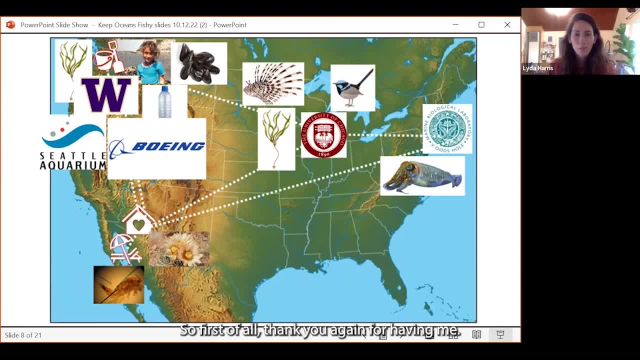 Yeah, so first of all, thank you again for having me. I wanted to explain kind of my background and my point of view. I'm from a place-based perspective, So this slide is quite jumbled, But I wanted to start off saying that I am from Tucson, Arizona. So in the bottom left-hand corner, that little house with a heart which is landlocked. 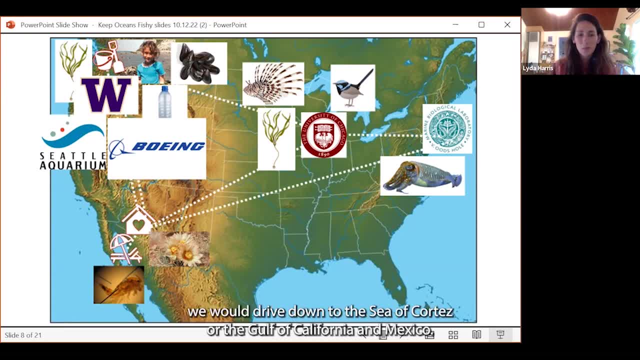 And I would take vacations down to, we would drive down to the Sea of Cortez or the Gulf of California in Mexico, And we would also go and visit my grandparents up in Whidbey Island just north of Seattle. And so those are the two kind of white outlined doodads at the bottom left and top left corners. 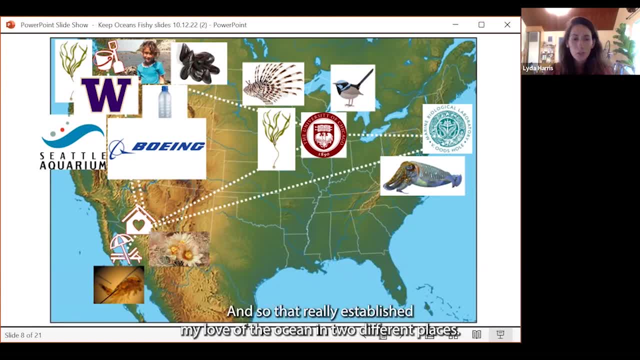 And so that really established my love of the ocean in two different places. So one was very warm waters in the Gulf of California and one was very cold, temperate waters in the Salish Sea, And from both of those places I just love looking under rocks, playing in the sand, swimming in the water. 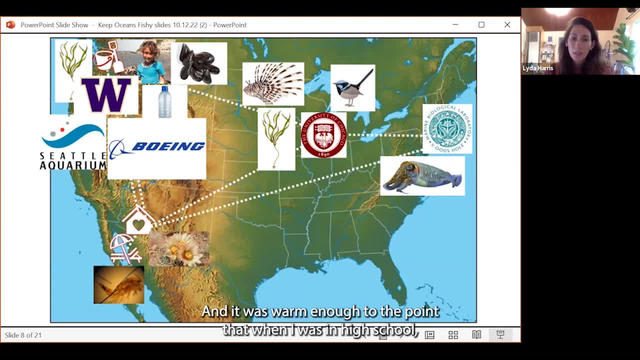 I'm very passionate about that, And so I took a couple of hours when I could and it was warm enough, to the point that when I was in high school, I did a science fair project based on copepods. so plankton in the Gulf of California. 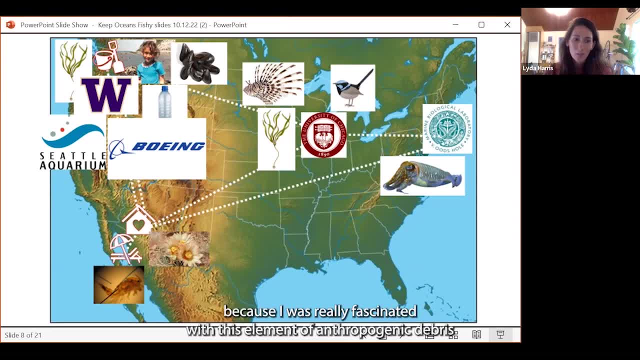 And they were, if they were ingesting plastics or not, because I was really fascinated with this element of anthropogenic debris, or like human-made debris in our natural environments. So from there that really informed what I wanted to do, kind of. 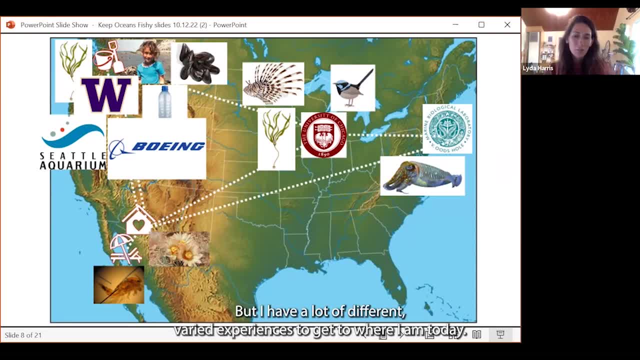 But I have a lot of time, different, varied experiences, to get to where I am today. So from there I went to college at the University of Chicago, another relatively landlocked state. We have the great lakes but nothing ocean. I was able to work my way into a lab studying algae and kelp that went out into Tatoosh Island. 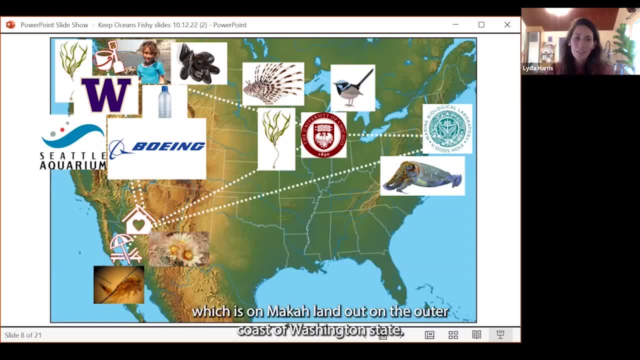 which is on McCall land out on the outer coast of Washington state, And so I went back to Washington, this place that I really loved, even though it was nice and cold, really cold during the summer. From there I went back to Chicago. I needed to be paid and the lab can no longer. 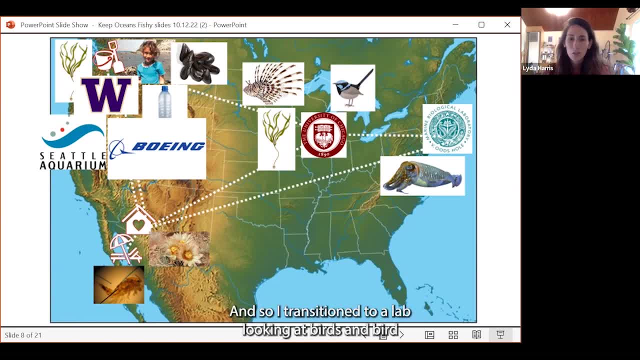 fund me to do any more work, And so I transitioned to a lab looking at birds and bird feathers, which I learned that I don't. I don't really like birds, So I got away from that and went into a lab at the Field Museum of Natural. 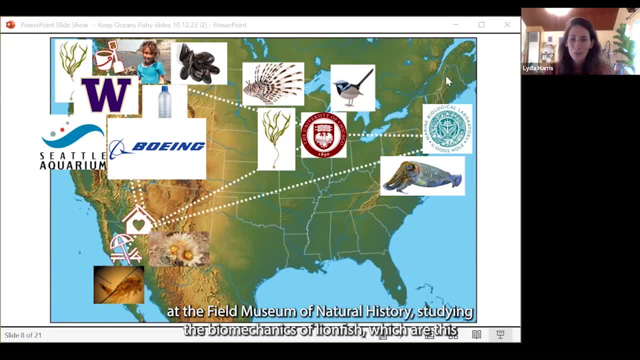 History, studying the biomechanics of lionfish, which are this very invasive fish in the Caribbean and the Atlantic that eat pretty much everything. So looking at how successful they are at eating, After college I went to the Marine Biological Laboratory out in Woods Hole. 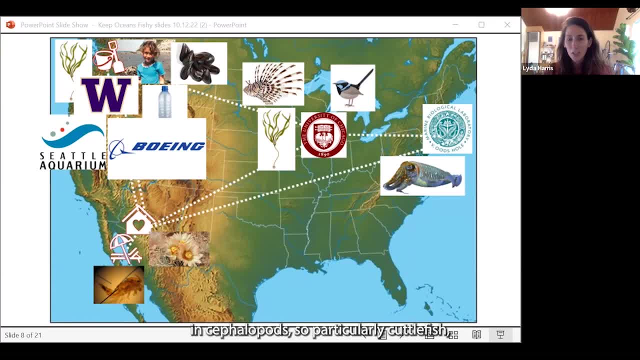 where I had an opportunity to study color change in cephalopods. So I started working on the biomechanics of lionfish, which is particularly cuttlefish, which gave me this perspective of how skin can change and how organisms can change to. 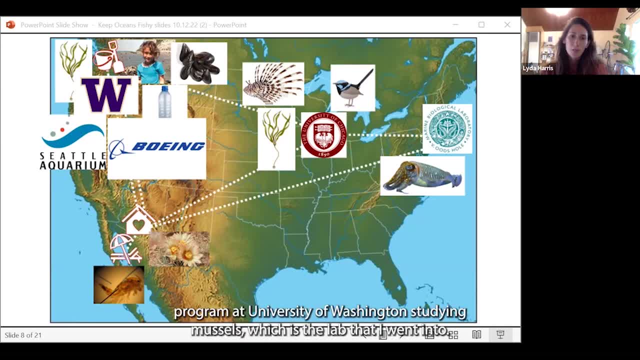 meet their environment, where they are in their habitat and their place. And then I started a PhD program at University of Washington studying mussels, which is the lab that I went into, And so I have this kind of unique perspective of biomechanics, natural history and ecology. 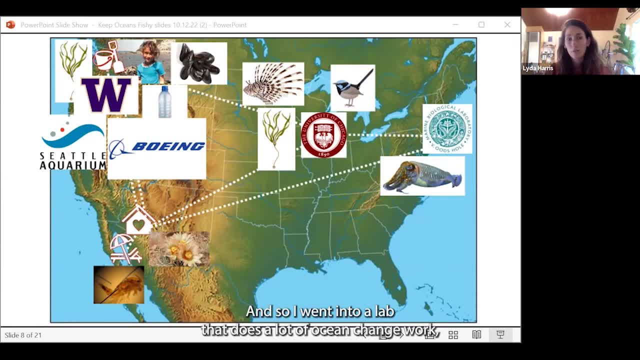 and adaptive change, And so I went into that lab and I found a lot of interesting things about it. I went into a lab that does a lot of ocean change work, And I was still really fascinated by this question of how people influence the environment, And so I brought with me my knowledge of plastics. 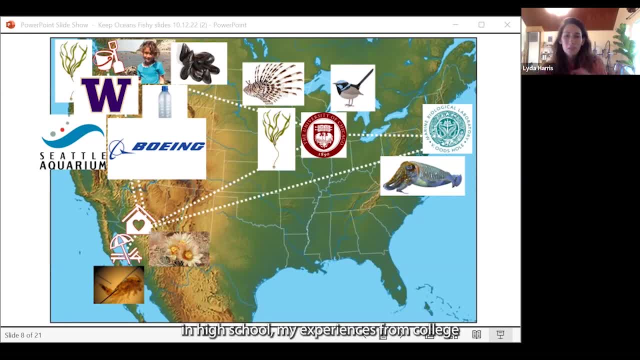 from when I did a science for project in high school, my experiences from college and from after college, as well as my love of the Pacific Northwest, And I studied how plastics degrade in the environment and also affect the physiology, biomechanics and different elements of organisms. 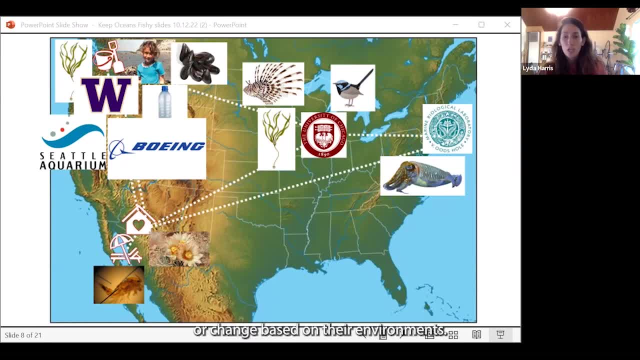 and how organisms can potentially adapt or change based on their environment. So after my PhD I went to the Seattle Aquarium and led their microplastic program and their clean seas program, really expanding what they did, And this was a wonderful opportunity to further my work and 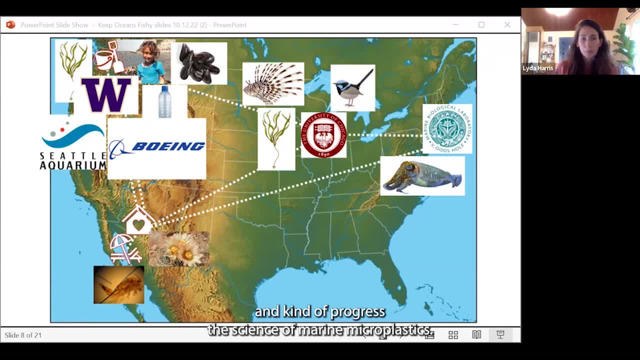 kind of progress- the science of marine microplastics- But I still wasn't quite getting that actionable change of how do we influence people's behavior and make the world a better place, I guess. So I'm switching to Boeing, actually in two days. I haven't started yet to work on behavioral change and working on their 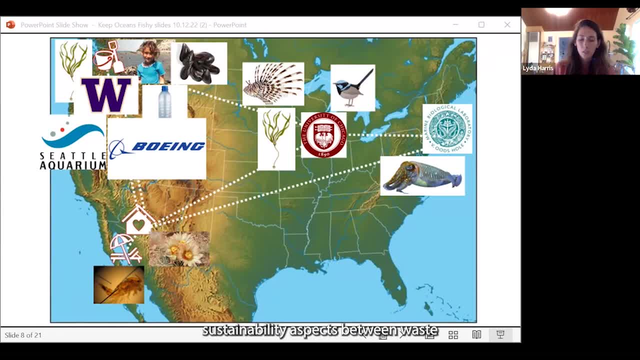 four main sustainability aspects between waste reduction, toxic waste, greenhouse gases and carbon- to really go inside the industry level and the corporate level to make a change, instead of waiting for policies to happen or waiting for other people to do it to really push this large. 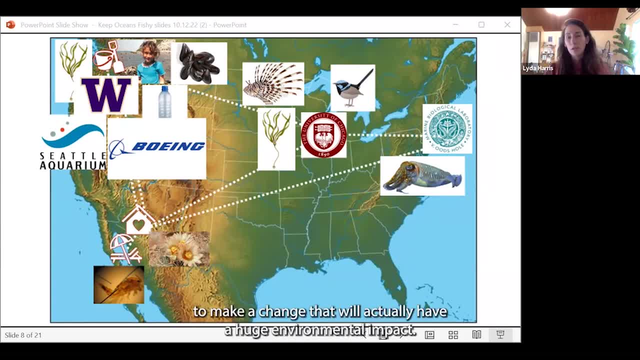 company that's in so many different places to make a change that will actually have a huge environmental impact. So that's kind of the perspective I'm coming from- Wonderful- And congratulations on your on your new role. I'm so glad that you've landed in the 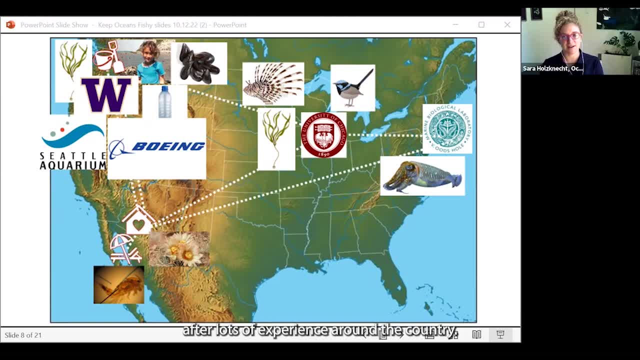 Pacific Northwest. after you know lots of experience around around the country And so there are increasingly more women starting careers in science And I'm curious: what is your experience as a woman in this field? Yeah, so I have found um. my initial positions I had were very 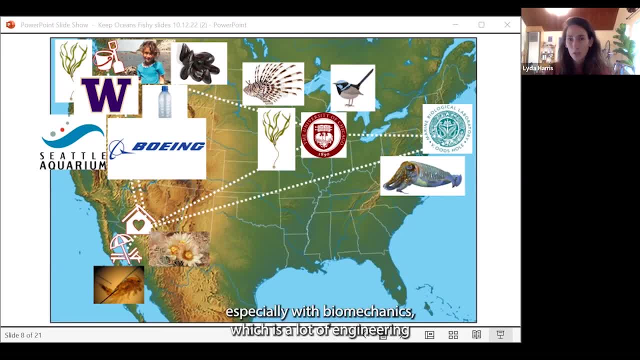 male, especially with biomechanics, which is a lot of engineering and physics, So there was that aspect of it. However, the more move into conservation and sustainability and waste reduction, the more women I work with, And so both my team at the Seattle Aquarium. 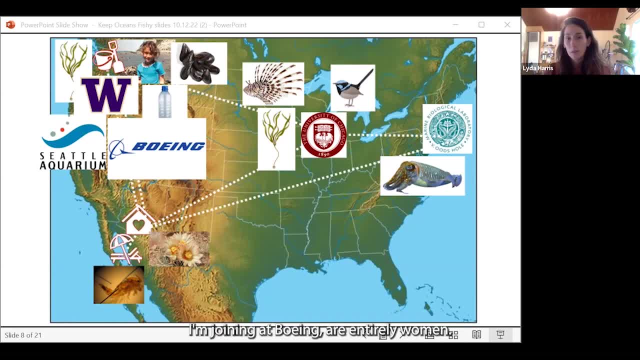 as well as the team I'm joining at Boeing are entirely women, And so I think it both leads a lot, shows a lot of empowerment that we have- and I love being on those teams- but it also highlights the need for increased diversity, both in terms of we need more than just women to care. 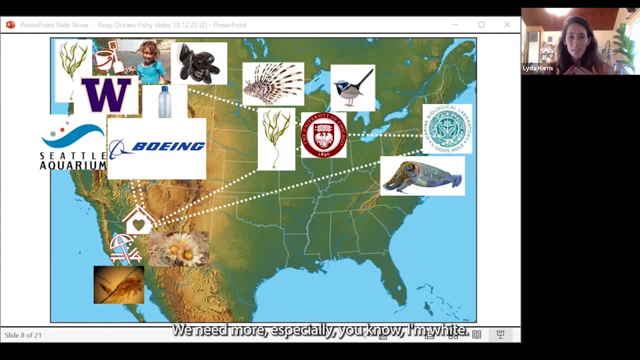 about this. we need more than especially. you know, I'm white, most of the team is white, and so we have a lot of white women that really care about this, and so I think, while it can be empowering, it also shows the lack of diversity in those spaces and the need to increase diversity in a lot of. 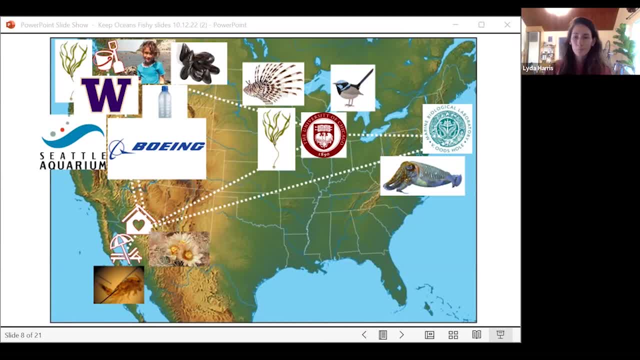 different sectors. Absolutely, thank you for naming that. that is so important. Yeah, so, as you know, Oceana is campaigning for healthy, abundant, sustainable fisheries policy and, based on your research, you know in a lot of different areas why are strong fisheries policies important. Yeah, so we've seen time and time again that as we have increased regulations of our fisheries, 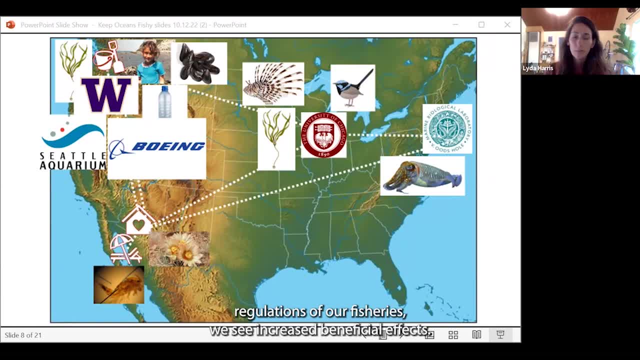 we see increased beneficial effects, and so, whether you're looking at marine protected areas or you're looking at specifically the catch that you're allowed in different regions, we're learning that we can't just go out and have a fish farm and we can't just go out and have a fish farm and we can't. 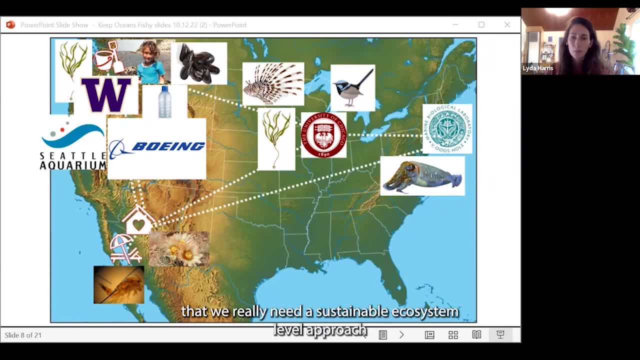 harvest everything that we really need: a sustainable ecosystem level approach and a really like a place-based approach that whatever works in Massachusetts or Maine is not going to work in California or Washington, necessarily, or Alaska, and that we need to come with those place-based approaches. we need to learn the ecosystems and once we do that, we can. we can. 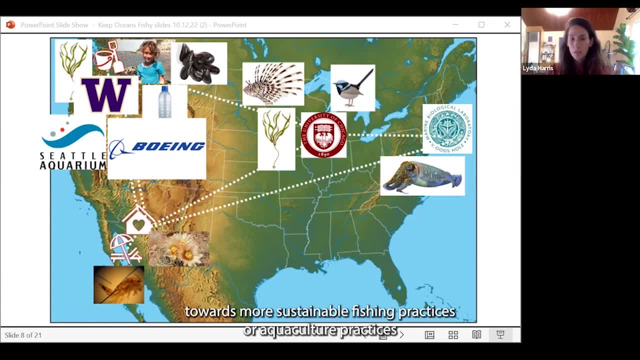 go towards more sustainable fishing practices, Our aquaculture practices, and really learn how the systems, the marine systems, can be sustainably harvested- Absolutely. thank you so much for that and thank you for joining today. If folks have more questions for Lyda, please do put them in the chat or in the Q&A and we will be doing a Q&A section at the end. 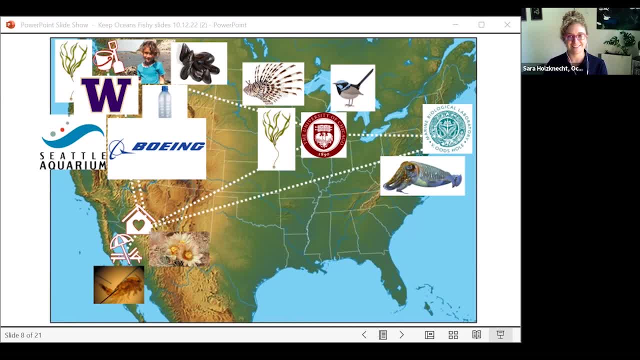 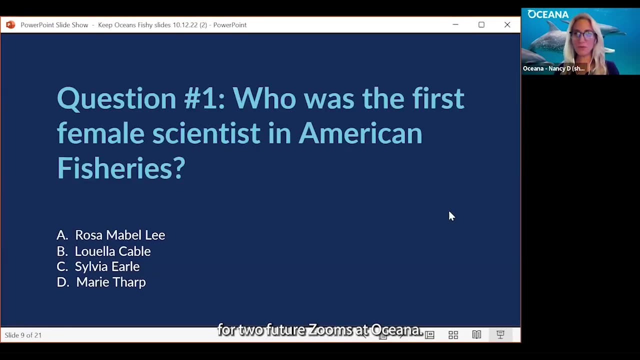 And potentially can ask questions And get those questions answered prior as well. I'm going to jump in. Thank you, Lyda. I have an idea already for two future Zooms at Oceana. I'm going to name the first one biomechanics of lionfish, and the second Zoom is going to be color changes- encephalopods. 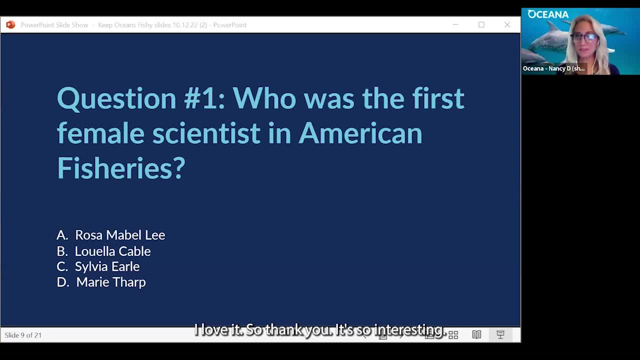 I am, I love it. So thank you, It's so interesting, And thank you, Thank you, And thank you again for joining us. So we're ready for our first poll. The question is: who was the first female scientist in American fisheries? 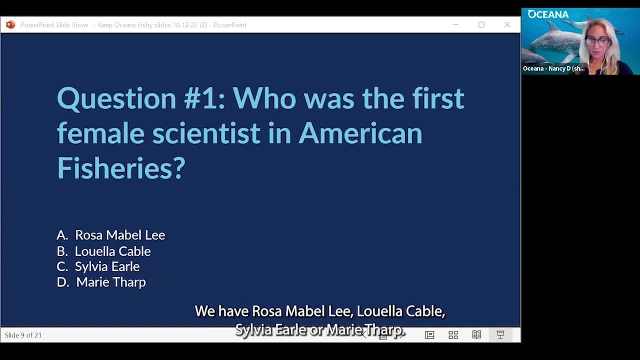 We have Rosa, Mabel Lee, Luella Cable, Sylvia Earle or Marie Tharp. We're going to leave this up for just a couple seconds. Give you all a chance. There should be a poll that pops up on your screen. 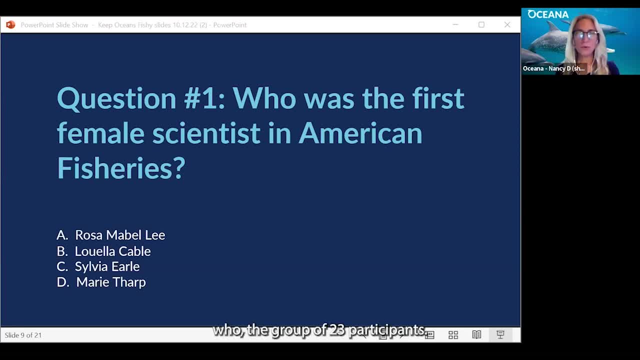 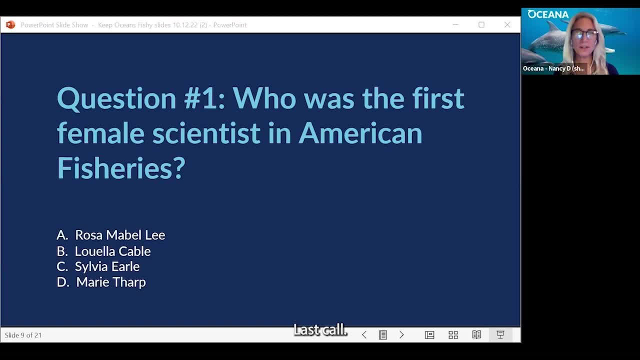 We've got. let's see, 11 out of 15 have participated. Anymore else Last call? All right, So we're going to end the poll And the answer is 27% of you got it right: It is Luella Cable. 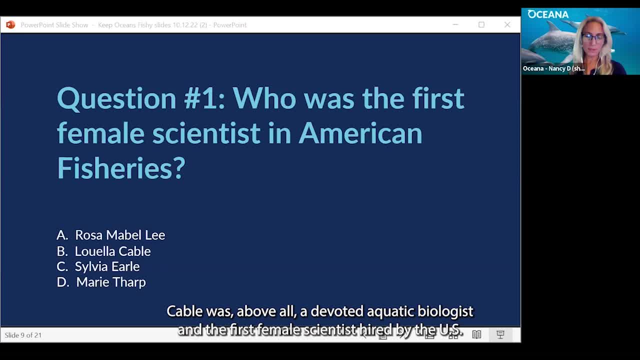 a devoted aquatic biologist and the first female scientist hired by the US Bureau of Fisheries, which was the predecessor of the US Fish and Wildlife Service in 1927.. So thank you for taking the poll. I think I shared the results. I'm going to close that out And back to Sarah for 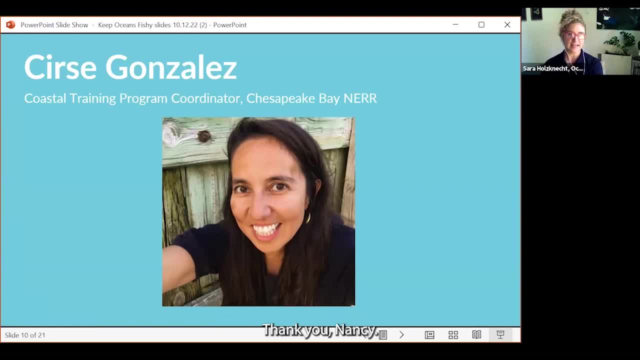 introducing our next speaker. Thank you, Nancy. At this point I'd like to introduce our next panelist, Circe Gonzalez. As Coastal Training Program Coordinator with the Chesapeake Bay National Estuarine Research Reserve in Virginia, Circe works on informing and empowering coastal 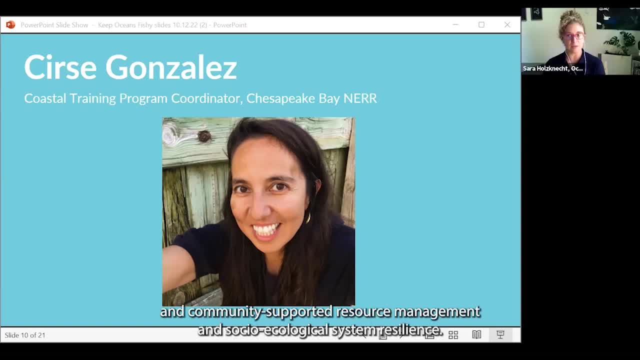 decision makers and fostering science-based and community-supported resource management and socio-ecological system resilience. Circe brings experience in communications and outreach, natural resource management, responsible recommendations and research. Circe is a member of the US Fish and Wildlife Service. 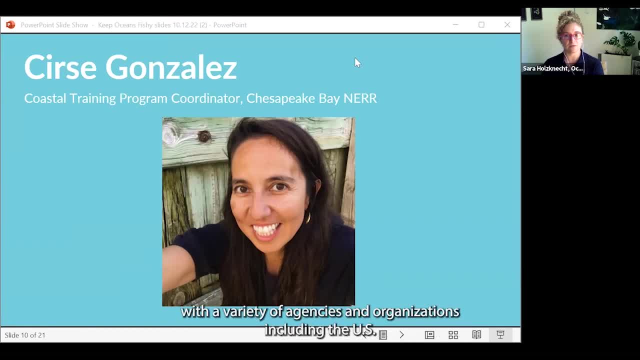 Recreation and Marine Ecology from her work and research with a variety of agencies and organizations, including the US Federal Recreation Council, where she served as Executive Director, NOAA's Office of National Marine Sanctuaries and five US Marine Laboratories While navigating. 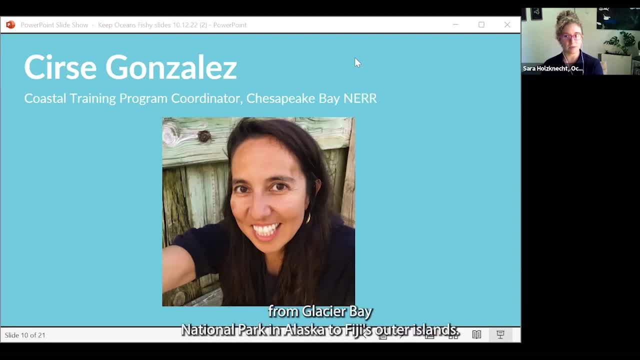 her career. Circe has lived and worked in geographies from Glacier Bay National Park in Alaska to Fiji's Outer Islands. Circe has a Bachelor of Science in Biology from Duke University and a Master of Marine Affairs from the University of Washington. Welcome Circe. 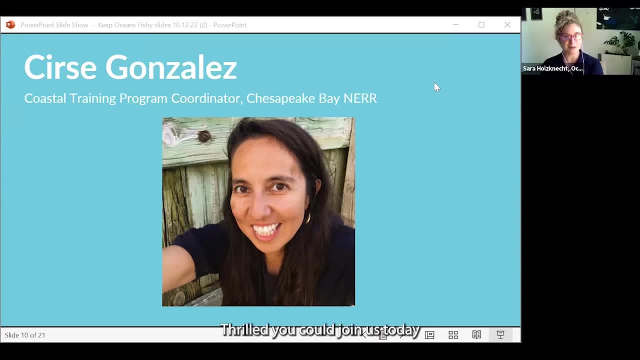 Thank you so much for having me here, Thrilled, thrilled. you could join us today. So it sounds like your work has taken you all over the world. Can you share a bit more about your journey? Oh gosh, yeah, I like to call this my 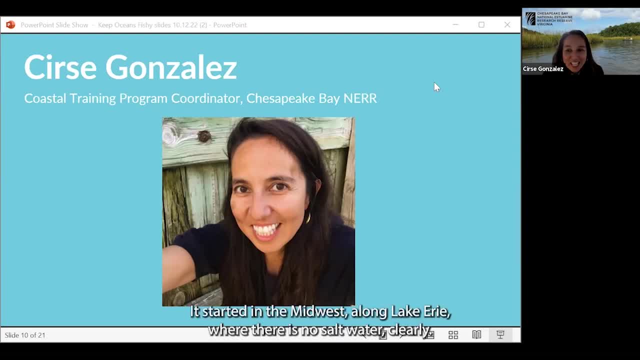 river of life. It started in the Midwest, along Lake Erie, where there is no salt water, clearly- and I want to actually circle back on this point, but I'll take you through. I I had all kinds of fantasies about being an FBI agent, an author. I ended up settling on 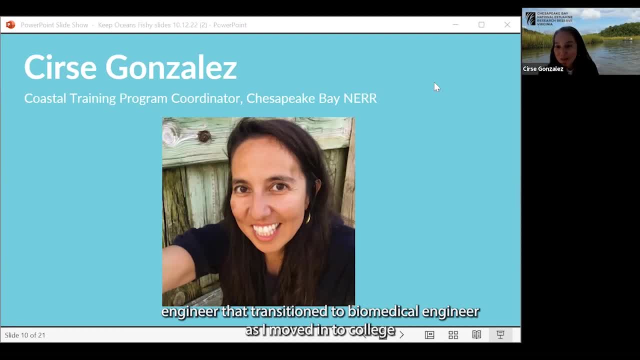 an aerospace engineer that transitioned to biomedical engineer. as I moved into college my first year, I discovered super quickly that that wasn't for me and I took to biology and instantly fell in love. I had amazing experiences as an undergrad, visiting multiple marine labs around the country doing phenomenal work on algae. 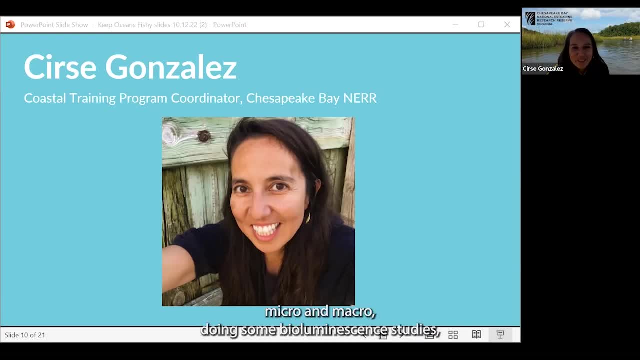 micro and macro, doing some bioluminescent studies, looking at the environment, and I was able to do a lot of research on algae, and I was able to do a lot of research on algae, and I was able to do a lot of research on algae. looking at larval crabs, which I still see in my dreams and in the clouds. 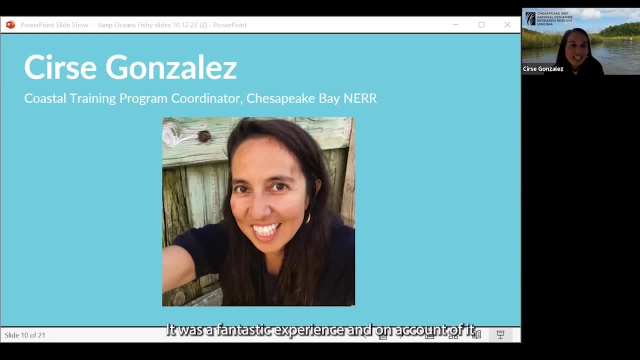 it was a fantastic experience and on account of it, I wanted to pursue marine biology. so I had it in my head that I would be doing a PhD after undergrad. but in between I wanted an international experience, something that was challenging, something that was foreign and something that would really help me grow. so I took to the Peace Corps, and that's. 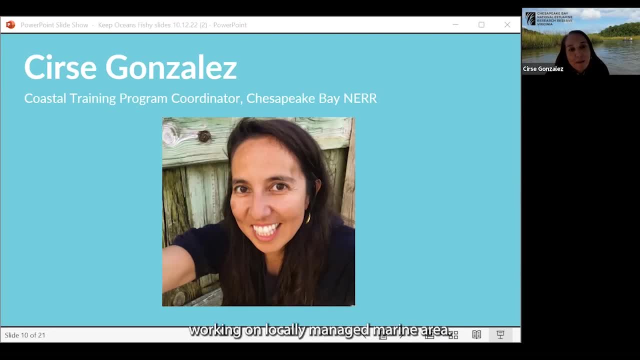 how I ended up in Fiji working on locally managed marine areas, and it wasn't long after that I decided I'm not going back for a PhD. I really want to work with the people on the grounds and and just be a little bit more applied, and I was able to do a lot of research on algae and 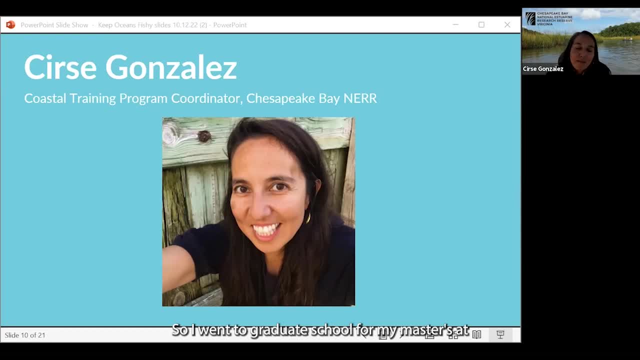 and just be a little bit more applied, and I was able to do a lot of research on algae. and and just be a little bit more applied, and I was able to do a lot of research on algae. and so I went to graduate school for my master's at, as you said, the University of Washington. 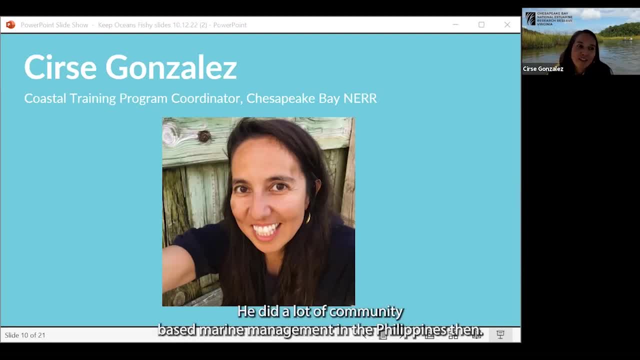 my advisor there was Patrick Christie. he did a lot of community-based marine management in the Philippines then, so my research for my master's is based there. after graduate school, I really wanted to pursue international work and ended up. after graduate school, I really wanted to pursue international work and ended up. 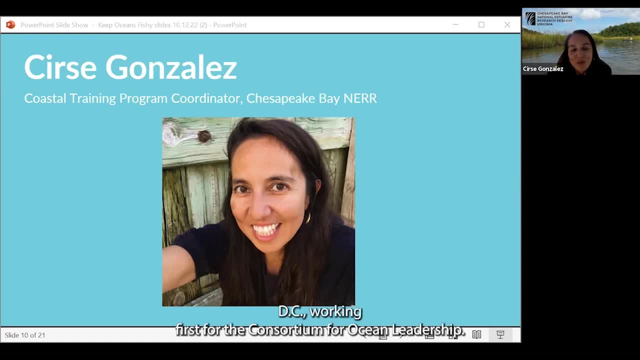 in Washington DC, working first for the Consortium for Ocean Leadership. I had an internship there and met somebody- through couch surfing of all places- that worked at the National Marine Sanctuaries. I had done a side study in grad school in concert with the tribes of the Pacific. 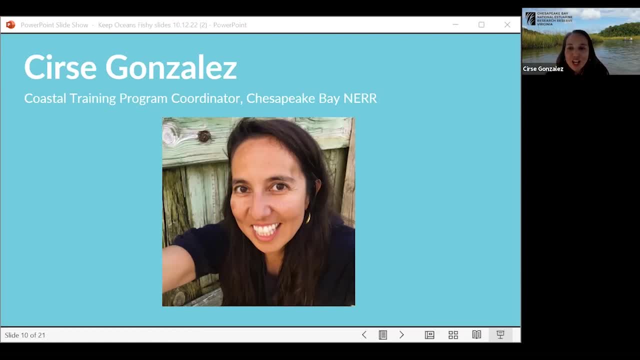 Northwest on the management of marine sanctuaries, so I was able to do a lot of research on the. this was something that we had talked about in this couch surfing experience, and this person kept me in mind when a position opened in her office and it was, you know, upwards from there. so I was in DC for 10 years before I decided that I needed a break from the headquarters, that I I really wanted to get my foot back in the game and I really wanted to get my foot back in the game. I really wanted to get my foot back in the game and I really wanted to get my foot back in the game. 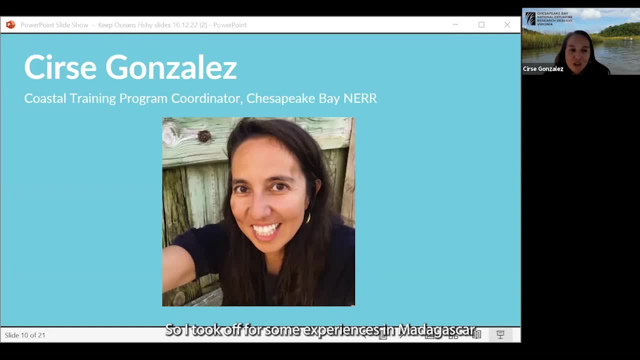 in international conservation. so I took off for some experiences in Madagascar and those helped me really decide that in fact domestic work is where I could make the most impact. and so I ended up back in the states working for the near system, doing what I wanted to on the ground in international spaces, but very much in a home. 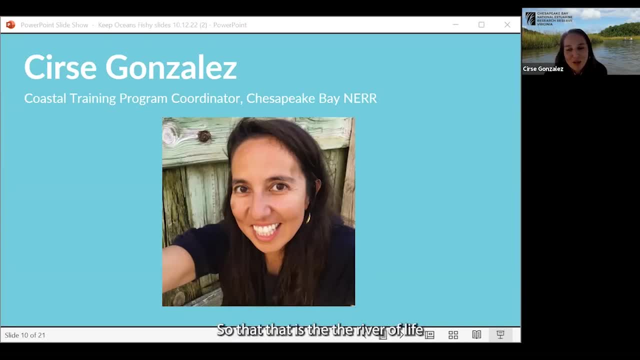 space where we're making great strides. So that that is the the river of life, but I wanted to throw in this fun tweet in the chat because I saw it earlier this year and it really had me thinking about. you know, what was it that I saw in my childhood in Lake Erie? that may have also 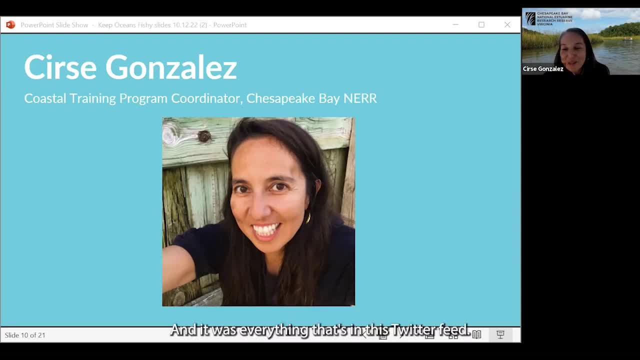 influenced my decision to pursue marine biology and it was everything that's in this project twitter feed. it was splash, it was mermaids, it was lisa frank, it was sea world, it was the voyage of the mimi. um, so i you know, if i know i'm preaching to the choir here, but, as i like to say, the choir 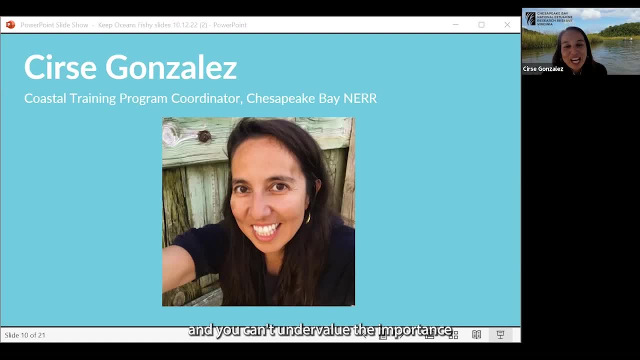 goes out and talks to the bands. um, you can't undervalue the importance of education at early ages. um, talk about impressionable and it all circles back. so there you have it. absolutely, it's so important and thank you for sharing. sharing that i love it. um, so it sounds like. 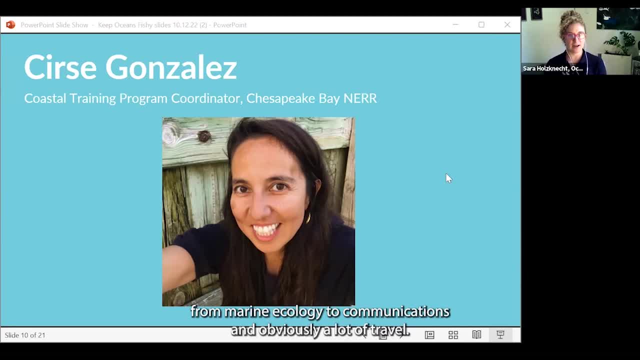 your work has encompassed many different areas, from marine ecology to communications and, obviously, a lot of travel. um, what advice would you give to young women who are maybe either thinking about going to school in marine science or just beginning their career in this field? oh sure, go for it. um, you know, explore opportunities. 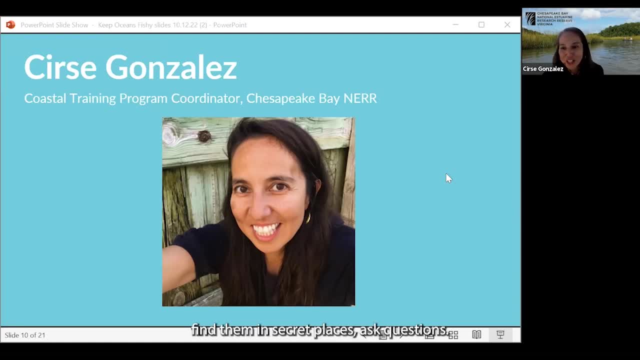 find them in secret places. ask questions, um, the more you ask, the more you know, right, and and there's a lot that's undiscovered out there- um, in terms of careers, in terms of opportunities and funding that will allow you to get to these places, i think that that remains an important 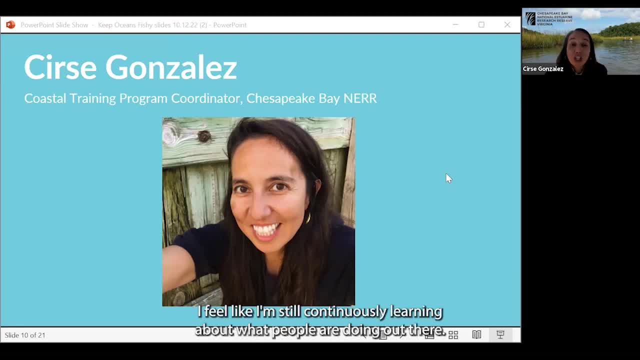 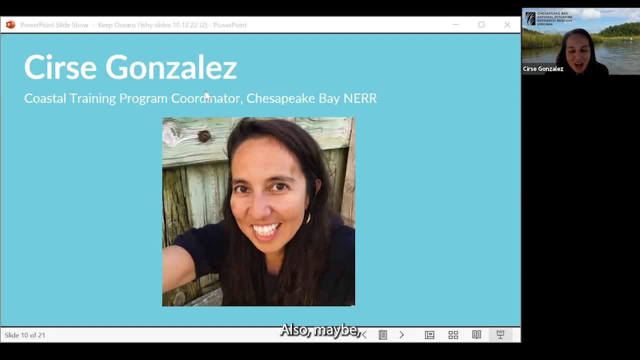 um, don't stop pursuing. also, maybe um you know, we have a lot of traditional notions about what success looks like. um you know it. it has had to do with title, it has had to do with salary, um, and i'd urge you to reconsider um, where you can find success in not only those things but 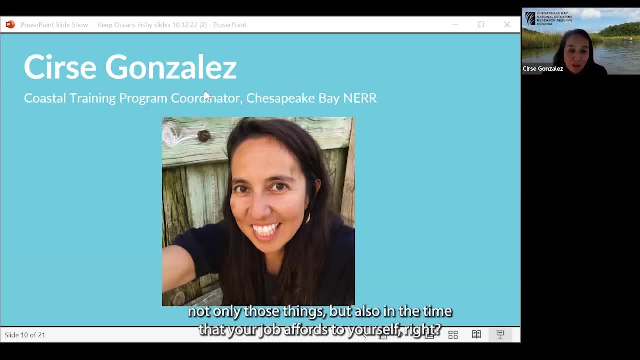 also in the time that your job affords to yourself right, the time that allows you to travel, to see new things, to um explore new ideas, um, there's a lot more balance there in in untraditional jobs and um it. you know you can't do it all by yourself. you can't do it all by yourself. you can't do it all by. 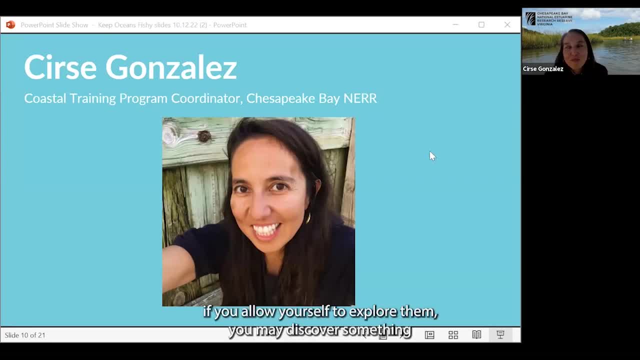 yourself you'll, if you allow yourself to explore them, you may discover something that you didn't know about yourself and that you, um, you really appreciate. so push back on those traditional notions. great advice. thank you so much for sharing and um and for joining us today. so, folks, um, please. 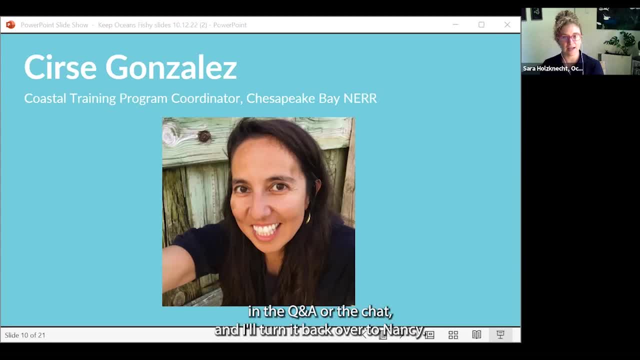 do ask seriously any questions you might have in the q a or the chat and i'll turn it back over to nancy. thank you, sarah and thank you, circe. i love your broad experience and, you know, just telling uh folks to take that first step and all those unexpected connections along the way, and i also 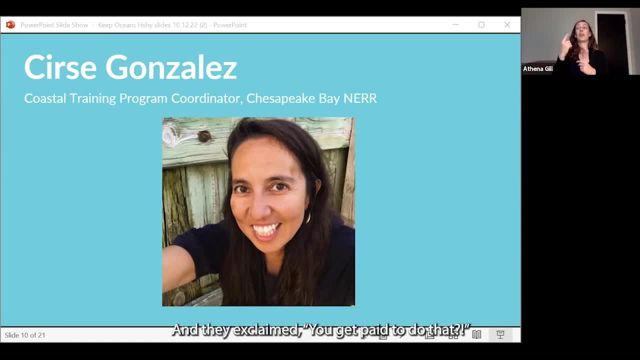 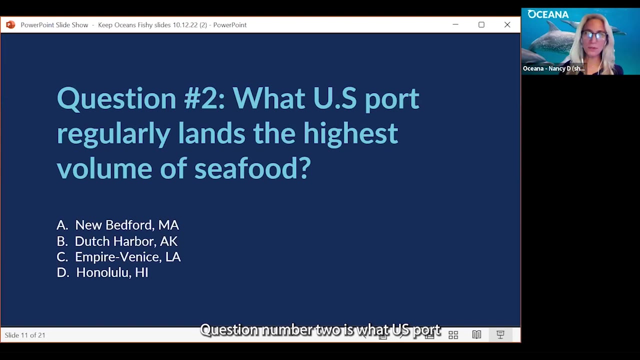 have a memory of telling someone what i do for oceana and they exclaimed: you get paid to do that. um, so, yeah, um, people's perception of success, uh, you just go for it, and i loved that advice. and now we are up for our next poll, question number two. 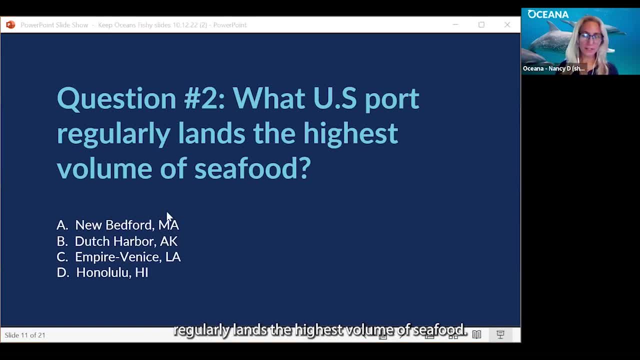 is what you think is the most important thing for you to do in your career. six was question one. we wanted to know your core values. six was the most important thing for you to do in your career. seven was the most important thing to do in your career. 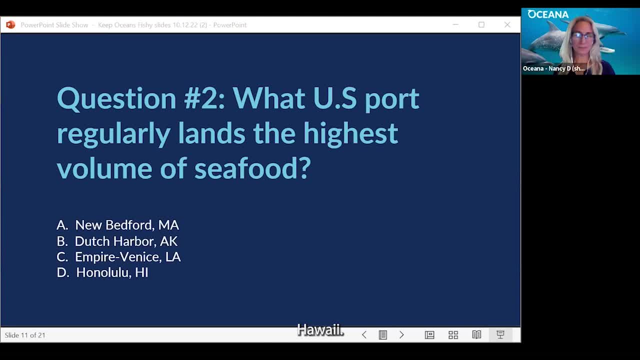 eight was to get the most out of your life. nine was the most important thing to do in your life. 10 was to find your best partner. 11 was to trade your life. 12 was to have a strong relationship with someone you love. Okay, a couple more seconds. 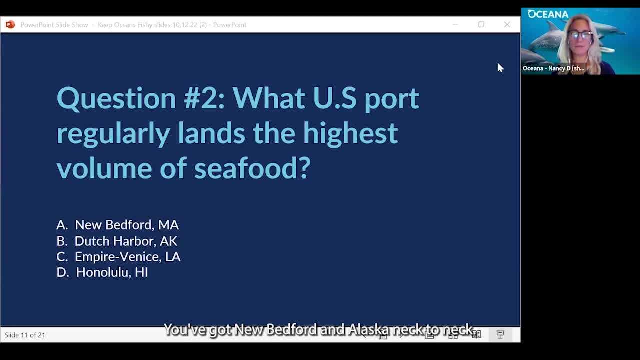 We've got New Bedford and Alaska neck to neck, So the answer to that question is B. for the 22nd- excuse me, 23rd- consecutive year, Dutch Harbor Alaska led the nation as the port with the highest volume of seafood landed with. 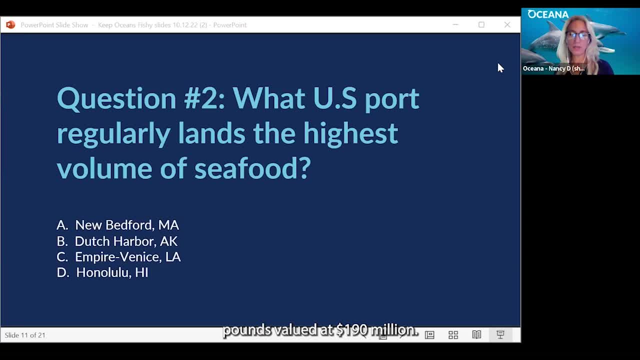 763 million pounds, valued at $190 million. But the follow-up answer is: the port of New Bedford in Massachusetts is America's number one in value. So Dutch Harbor, Alaska, was 190 million. In New Bedford, it's nearly 50 million pounds of sea scallops landed there, but they're valued at. 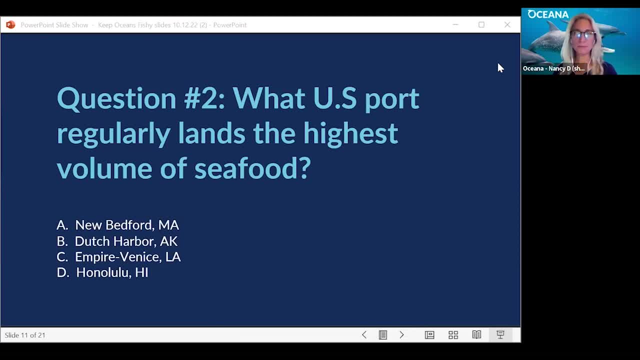 $3.5 million. So that's the answer to that question: $369 million, that comes into New Bedford. So great answers, folks, And we're going to move on. I'm going to pass the mic over to Anna, who's going to introduce our next speaker. Thanks, Anna. 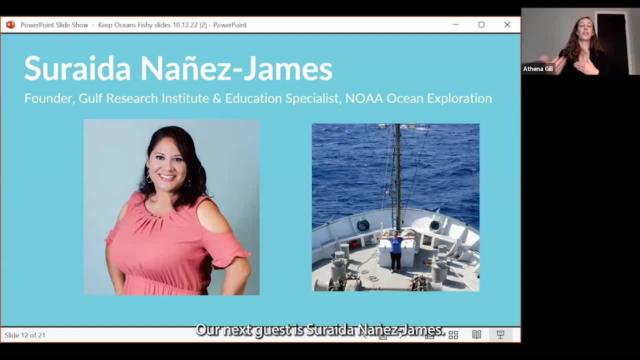 Thank you. Our next guest is Sarita Nanez-James. Sarita has been in the field of science and education for over 20 years, working in academia, for nonprofits, schools and the Texas State Aquarium. As an education specialist with NOAA Ocean Exploration, she's helped develop and lead. 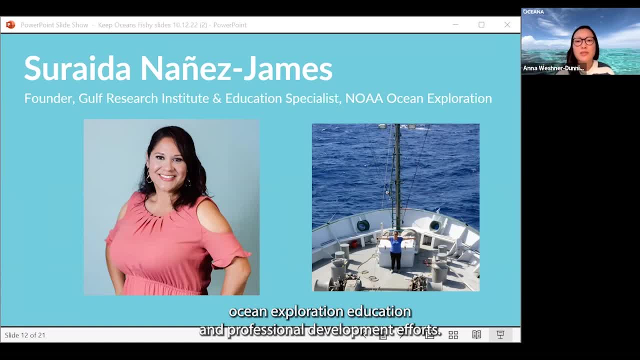 ocean exploration, education, professional development efforts. She is also a proud founder and CEO of the Gulf Reach Institute, which is a nonprofit dedicated to innovative and inclusive STEM, health and advocacy programming focused in the Gulf of Mexico and our oceans. The Gulf of Mexico is her home and her community and is why she's dedicated. 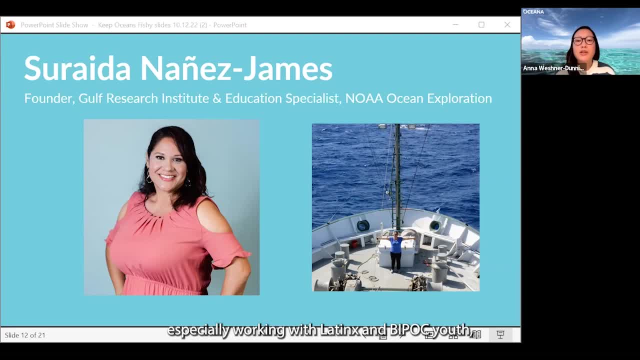 to giving back, especially working with Latinx and bilingual students, So I'm going to pass the mic over to Sarita Nanez-James, who's going to introduce our next guest. Thank you so much, Anna, for the introduction, and just a pleasure to be here amongst all these. 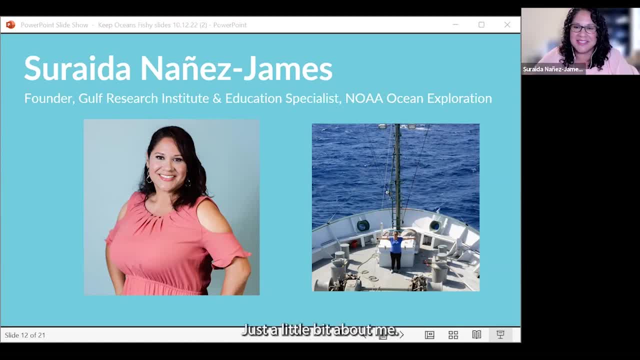 amazing women in fisheries. Just a little bit about me. So you heard a little bit about my background, but looking at where I started off, So I decided I wanted to be. I used to watch a lot of Discovery channels and that was my go-to every time. So I'm going to pass the mic over to. 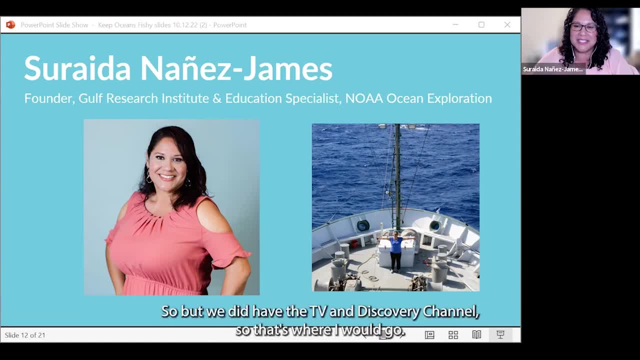 Sarita Nanez-James. So we didn't have very much growing up, but we did have the TV and Discovery channels. so that's where I would go. So we'd go outside, but at the same time we would see all. 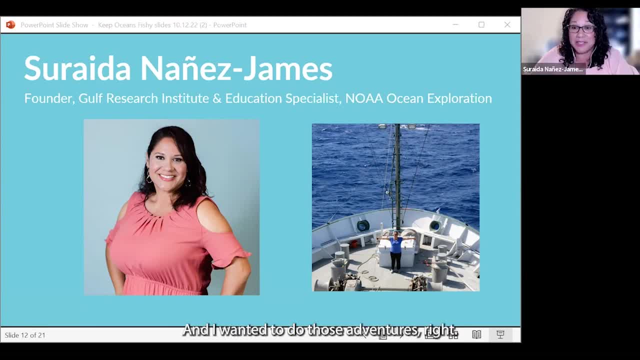 these amazing adventures on TV and I wanted to do those adventures right, So really dedicated myself to education and wanted to be a marine biologist since I was 12. So I would say. and I wanted to be a teacher and apparently a model too. So those three combinations, if you can. 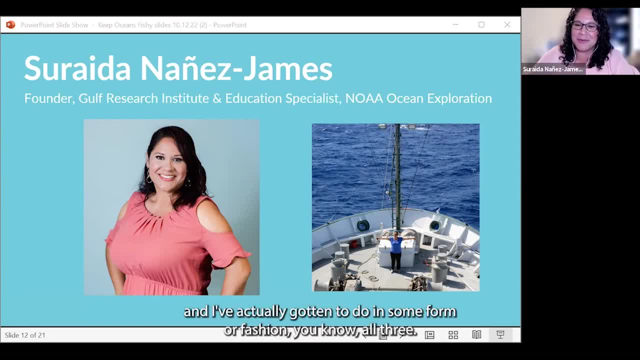 believe that, And I've actually gotten to be a marine biologist since I was 12. So I've been in some form or fashion. you know all three. So I got to become a marine biologist. I am still an educator, a lifelong educator, and through some community things I've modeled some outfits. So 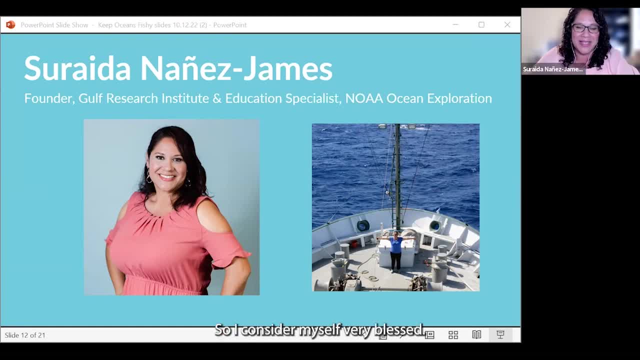 I got to do all three of those childhood dreams, So I consider myself very blessed. But just looking back, my first exposure really to the ocean, my love for water and my connection to water came from, you know, in the place actually that I live now. 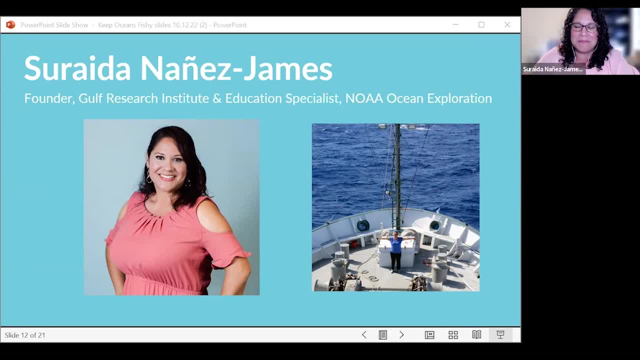 So I'm originally from San Antonio, Texas here, and we had lakes, So we went camping and a lot of outdoor things And you know, back in the days when my abuela would say: you come back when it's. 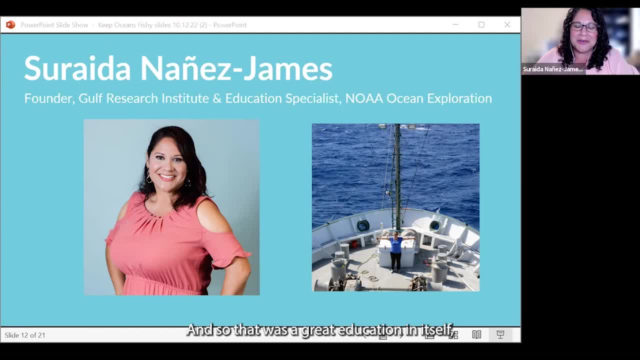 time to eat, So you spend your time outside, And so that was a great education in itself: just exploring nature and really appreciating it for its simplicity and complexity all at once, And so I was the first person in my family to graduate. 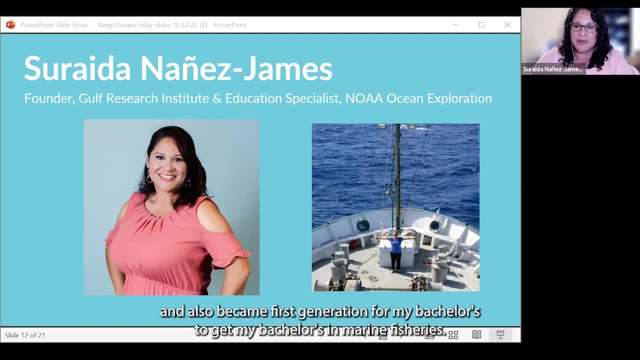 from high school and also became first generation for my bachelor's- to get my bachelor's in marine fisheries, I think some other folks you know they had the journey too. I wanted to do mammals and my first marine mammal class decided that that again. I've heard this before in all of the 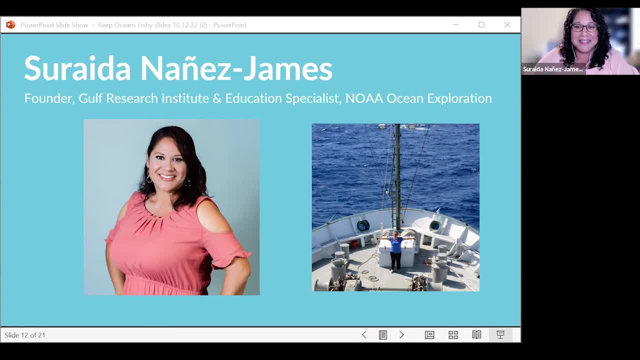 talk from the panelists that that was not for me, But took a fisheries class and fell in love with it And was able to. my first job was working at NOAA- at a NOAA business, and I was able to do that too. So been doing that for three years. and garlic- I don't know why I don't. 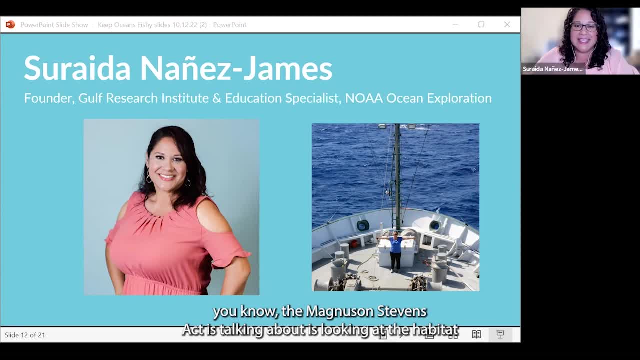 know why I have my own business, But yeah, it's been a really different time. And then I was able to join the SPPF — the Pacific and Fisheries Ecology Lab — and really doing really what you know the Magnus and Steven's act is talking about Is looking at the habitat. that 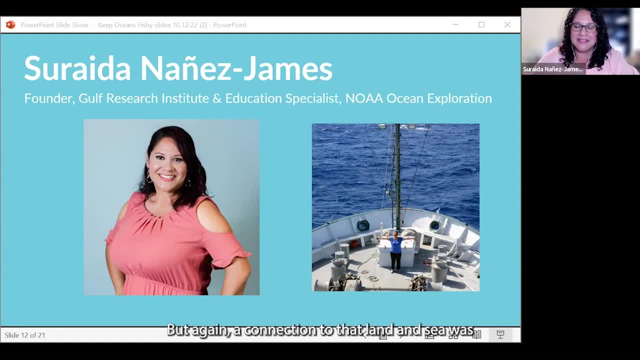 really provides the home and the shelter for the fisheries that we depend on. But again, a connection to that land and sea was what really kind of fueled my passion for it. And, like you said, Ana, I have a heart for the Gulf for sure. This is my home, And working with just Gulf 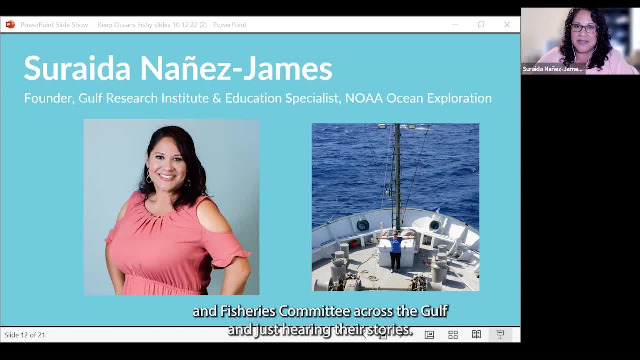 communities and fisheries community across the gulf and just hearing their stories, uh, anyone from you know the jin shakta. and in louisiana, to the vietnamese communities, um, and also hispanic communities, shrimpers, um, that all depend on on these fisheries for their livelihood. uh, was really. 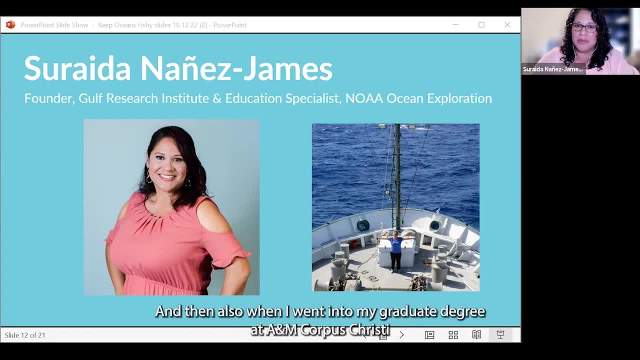 eye-opening as an undergraduate student and then also when i went into my graduate degree at a and corpus christi um, so really learning how to listen, how the different regulations affected them, um who supported what and and really looking to see beyond um what that meant for them right. 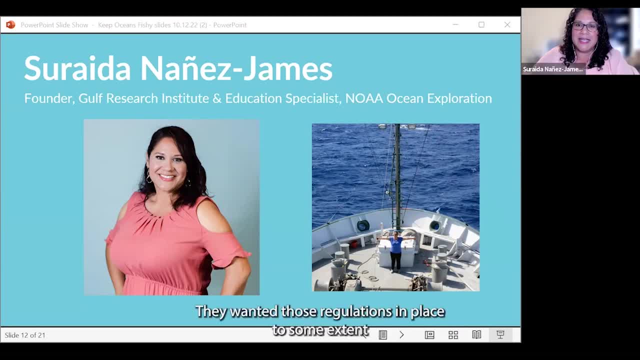 that's, it was their livelihood. at the same time they had they wanted those regulations in place, to some extent because it did help them to regulate and preserve what they depended on, but at the same time, you know, you know at really incorporating their knowledge and what they knew about fisheries, ecology especially here. 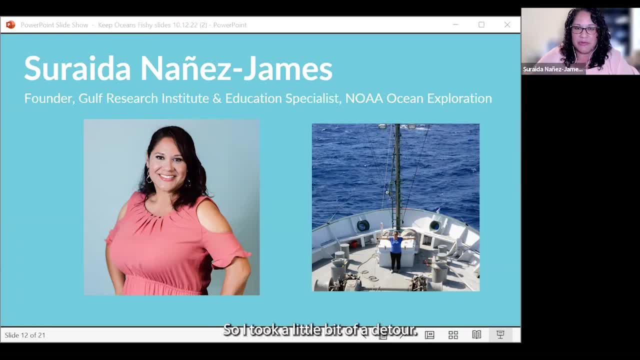 in the gulf. so i took a little bit about a detour. so i i did fisheries ecology for a while and then i went into restoration ecology, so looking again at those uh habitats and really working to conserve and preserve those habitats. um traveled a couple of uh, you know, fulfilling 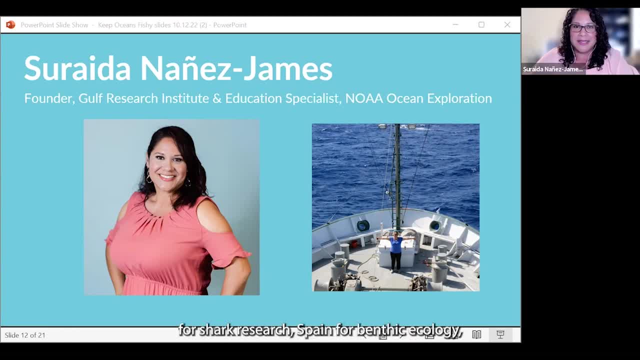 those dreams: going to south africa for shark research, um spain and other uh, for benthic ecology and just looking at different areas of things that i've really enjoyed doing. so i always say i look at the little tiniest things, the benthic, the worms that nobody looks likes to look at um, and then how? 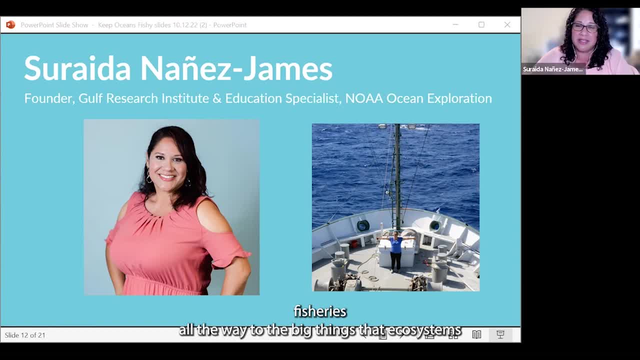 those really affect fisheries all the way to to the big things, the ecosystems that you know we fight so hard to preserve. but one of my biggest passions, i think- and you'll see it here- is just learning and teaching others. and, uh, one of our other panelists talked about representation. 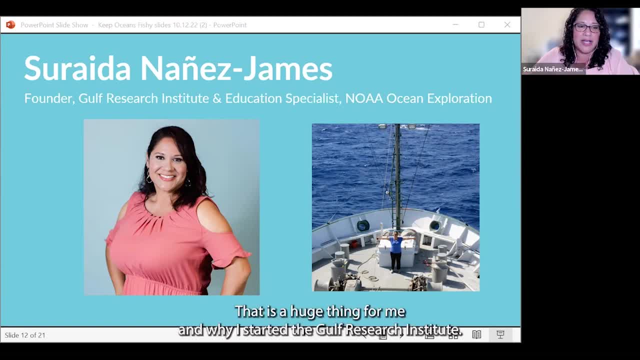 that is a huge thing for me. uh, and why i started the gopher each institute. we, we wanted a platform. we always say sometimes we get tired of waiting for to get invited to the table, so we made our own this time and so everybody's invited this time. um, and the gopher each institute? uh, research. 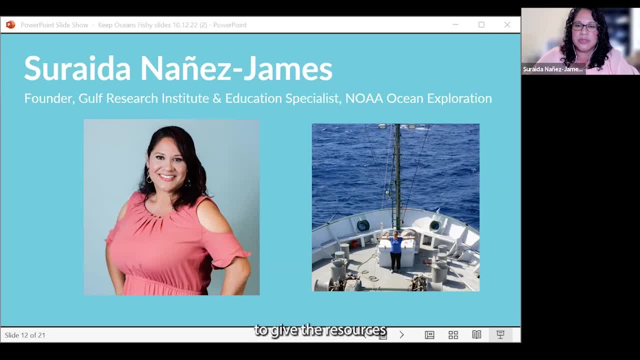 institute really focuses on trying to give to the people who are going to be involved in the um the resources that communities need um and then also learning from those communities at once. we do focus a lot of our focuses on youth and youth empowerment. uh, our board members are 19. 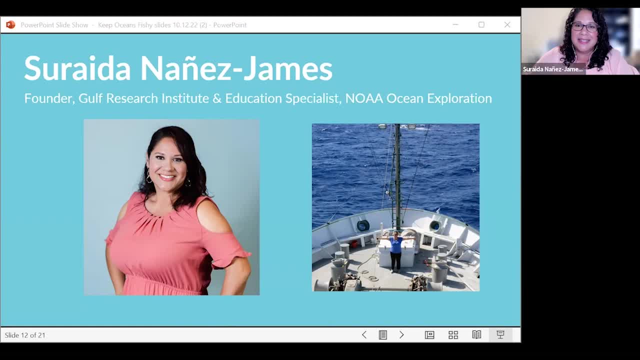 are for youth engagement, or 19 and 22, and i can tell you that they've taught me a whole lot as well. um, they work a lot on the climate change climate summit here in the gulf of mexico. uh, uniting our youth not just in the us but in the global climate change climate summit here in. 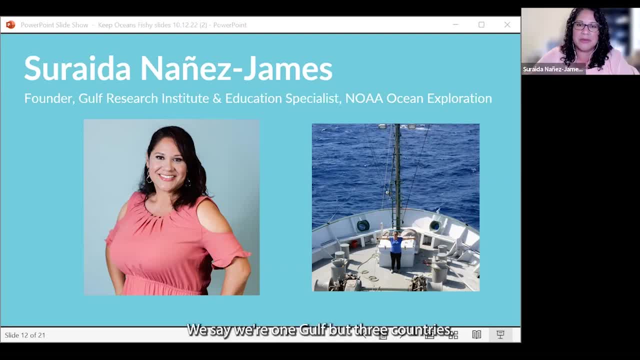 the us, but also in cuba and in mexico. uh, we say we're one gulf but three countries, so we have to look at management across borders. um, we always laugh and say that we can have all the borders we want, but the fish aren't going to care, they're going to go wherever they want, the sharks included. 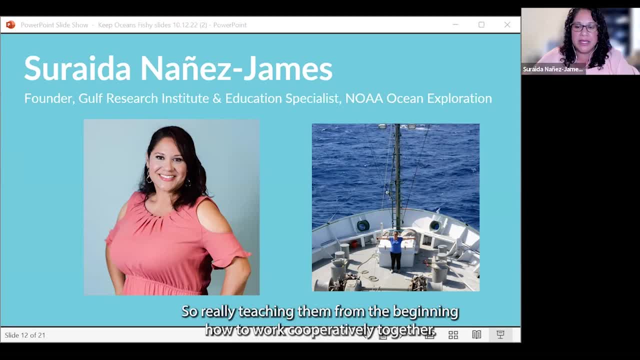 and then how do we manage that? so really teaching them, um, from the beginning, how to work cooperatively together, uh, and so that's, that's been the most fun part. you know there's the ceo part is kind of the hard part, but you know, uh, having having them or being part of their journey in 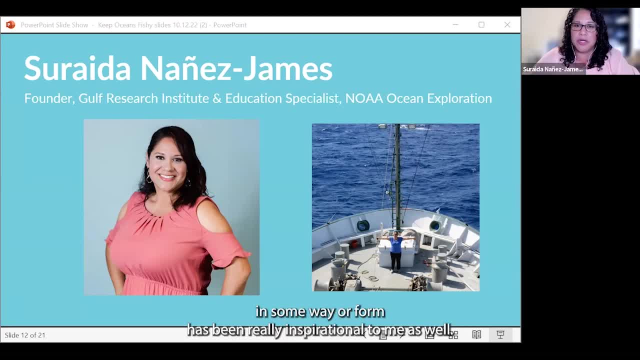 some way or form has been really inspirational to me as well, and i now work for noah ocean exploration. as education specialists i produce uh lessons and looking for professional development and then looking for other ways also to include more of a cultural pedagogy in there. 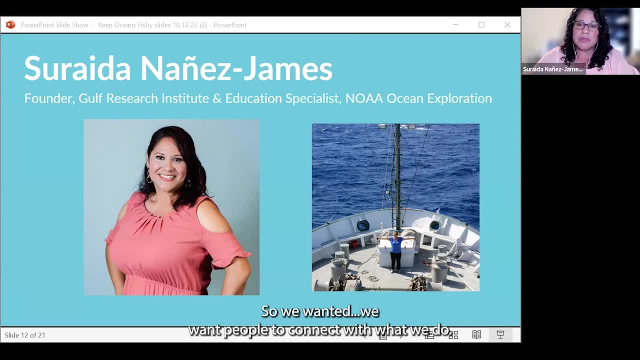 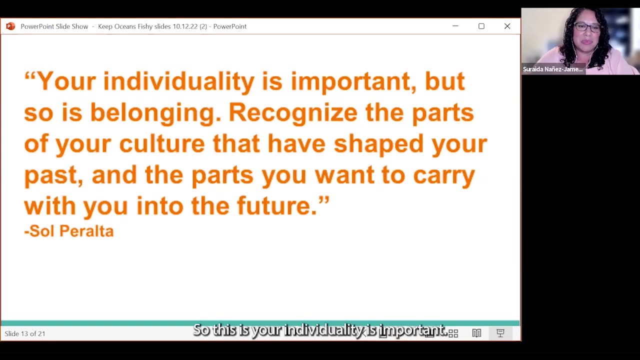 as well. so we want it to. we want people to connect with what we do. so that's one thing. uh, oh, the slides. yes, sorry, i forgot just in the slides. you can advance it if you like. um, so it says your, your individuality, is important. i loved this quote, but so is 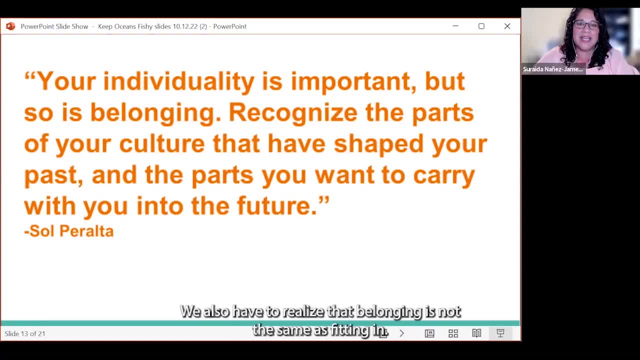 belonging. uh, we also have to realize that belonging is not the same as fitting in. i think for a long time we tried to fit in and that's that's not the same. uh, we recognize the parts of our culture that have shaped us in the past and that's the parts that we want to carry uh with us in the future, and i thought this was 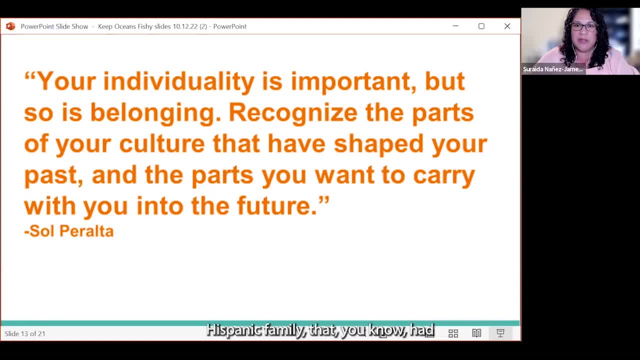 important because i i do come from a very traditional family, hispanic family, that, um, you know, had some different takes on me being in the field, especially in fisheries, ecology. uh, a lot of times being the only woman in the field, uh, that was kind of frowned upon like a taboo. 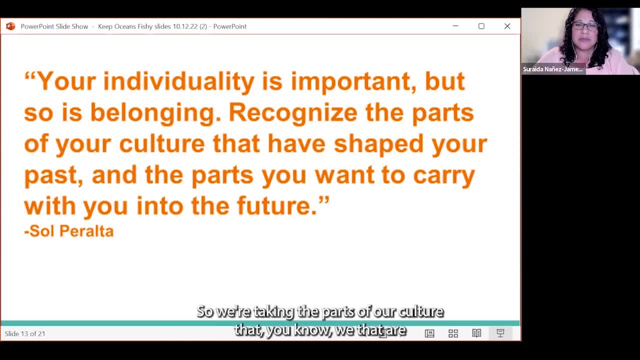 but at the same parts we say that we're evolving. so we're taking the parts of our culture that you know, we, that are conducive to the future, and we're taking the parts of our culture that are conducive to us, that talk to us in this generation, and then taking that forward as we. 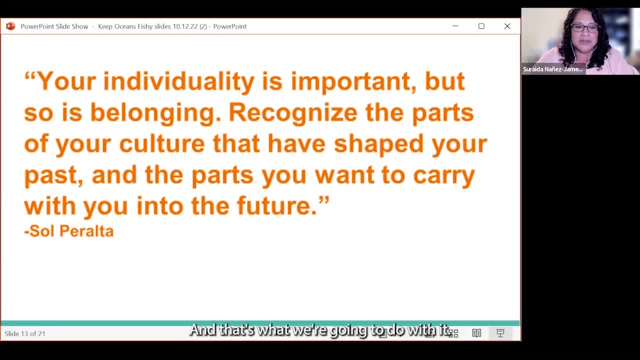 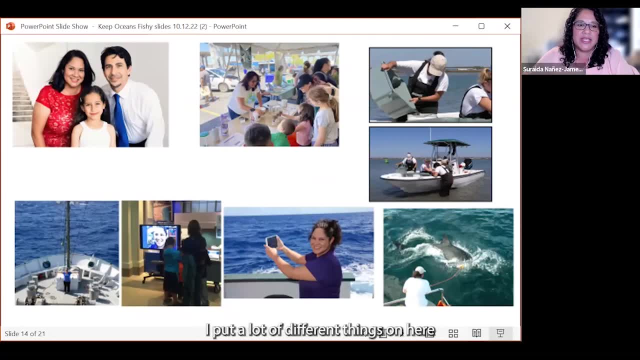 evolve, um, in this community, and that's what we're, that's what we're going to do with it. uh, can you go to the next slide? i don't want to take up too much time. i put a, i put a lot of different things on here because, uh, i like to say we're, we're not just one thing. so i am a wife, i am. 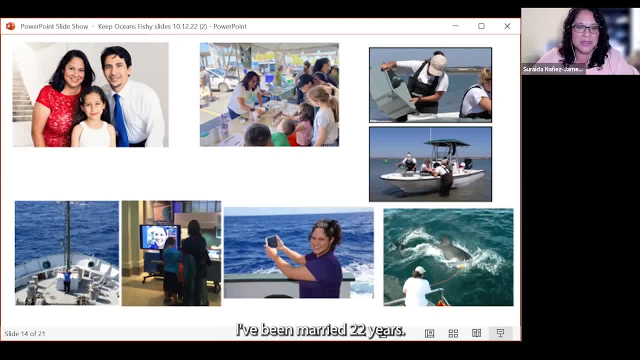 a mother. i have an 11 year old daughter. i've been married 22 years. i'm an educator- uh, i've taught in schools, uh, informally, and i've been a teacher for a long time, and i've been a teacher for a long time and formally. i love all my students. uh, i feel quite old sometimes when they're getting their. 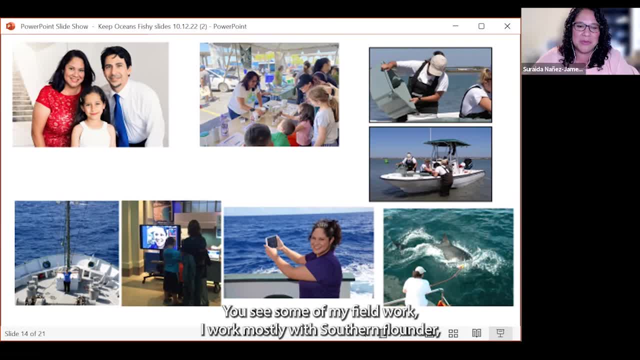 master's degrees now. uh, you see. so my field work. i work mostly with southern flounder, which is commercially and recreationally important. here in in texas i've worked with great whites. i've also sailed a lot on many of the ships looking at benthic- uh, excuse me, bathymetry and mapping. 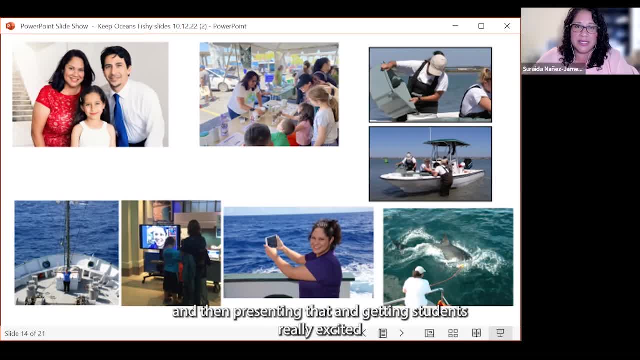 the seafloor and then presenting that and getting students really excited, um, about just the ocean in general and just why they should protect it and how to connect. and that includes making presentations in spanish to some of the students who predominantly spoke spanish. so that's kind of my life in a nutshell. uh, my passions, quickly you know, sharing with all of you. 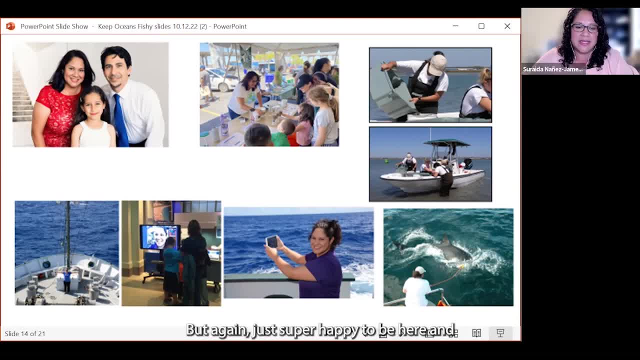 but again, just super happy to be here and, um, just honored to listen to some of the other folks that are going to be on here as well. thank you so much. yeah, thank you so much, sarita. it's really nice to hear your story and i appreciate you sharing. 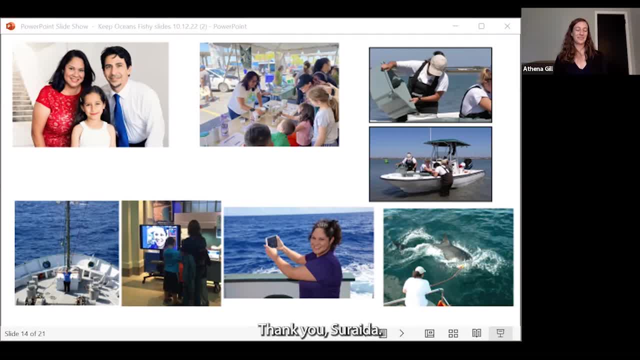 thank you so much, anna. thank you, sarina, also just impressed that you knew since age 12 what you wanted to be. you are not just a beautiful model, but a role model, and i loved hearing about the youth engagement, which i think is so important and often overlooked. so thank you again. 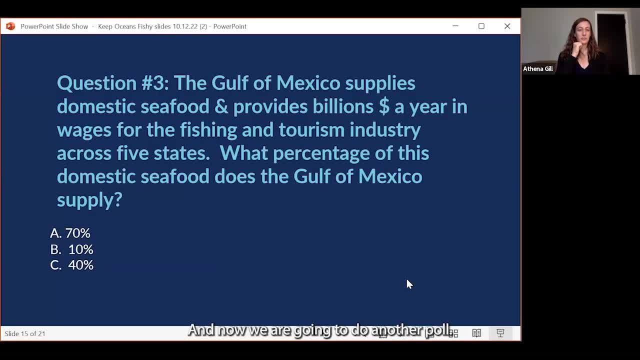 and now we are going to do another poll. so question number three: the gulf of mexico supplies domestic seafood and provides billions of dollars a year in wages for fishing and tourism industries across five states. what percentage of this domestic seafood does the gulf of mexico supply? 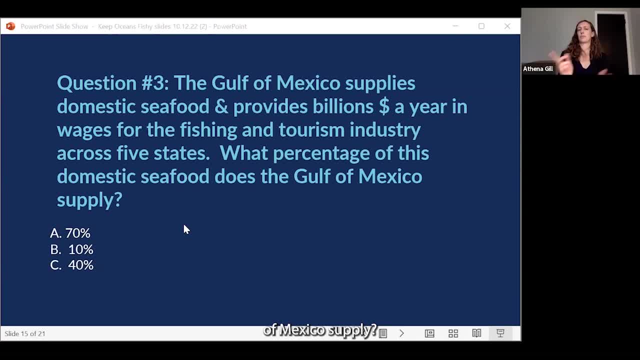 give a couple minutes, all right. so the correct answer is 40. more than 40 is domestic seafood. the gulf of mexico supplies as far as wages for the fishing and tourism industries across those five states. thank you for taking that poll and let me close that out. um. next up, we have an interview done. 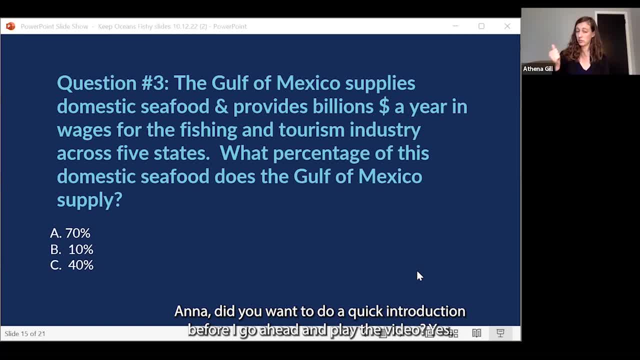 with anna. um. anna, did you want to do a quick um introduction before i go ahead and play the video? yes, so unfortunately emily could not be here live, but we will um stream her interview in just a second. our other panelist was emily sellinger. she was born and raised in freeport, maine, and is a water. 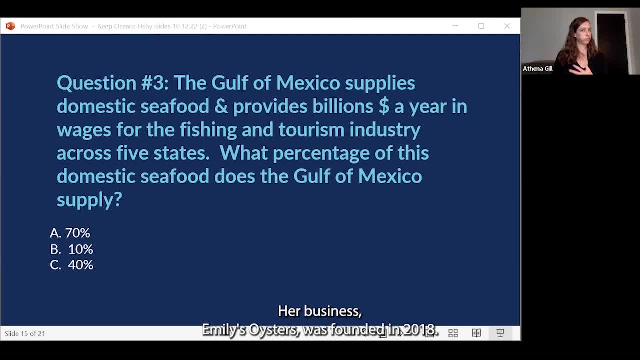 woman through and through her business. emily's oysters was founded in 2018 and it's a small scale woman-owned uh oyster farm in freeport, maine, where their company's goal is stewardship for health and well-being, and so i'm going to take a look at a little bit about that a little bit. 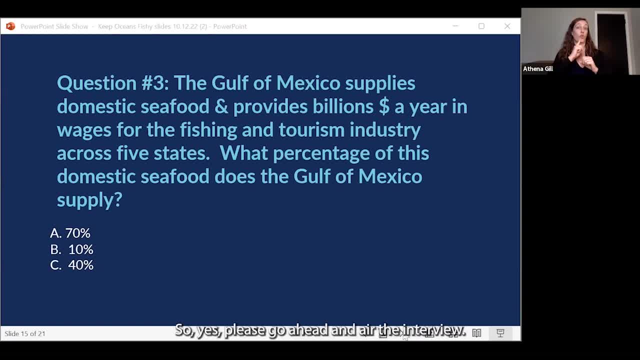 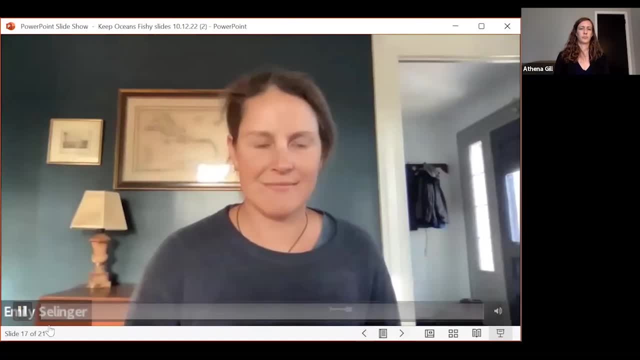 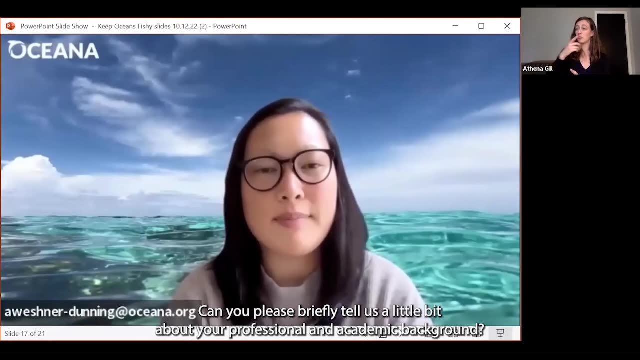 being of the ocean. So, yes, please go ahead and air the interview. Hi, Emily, thank you so much for joining us today. Can you please briefly tell us a little bit about your professional and academic background? Sure, Um, well, my academic background is highly unrelated. 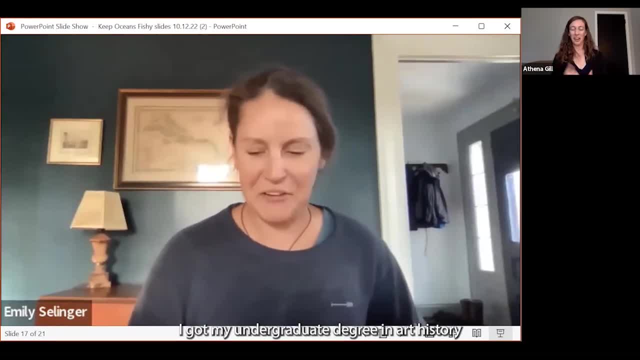 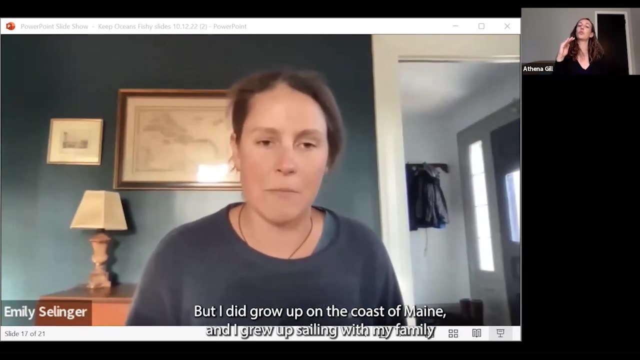 to what I do for work now. I got my undergraduate degree in art history and studio art and music And yeah, that has not really impacted what I do now. But I did grow up on the coast of Maine and I grew up sailing with my family and teaching. 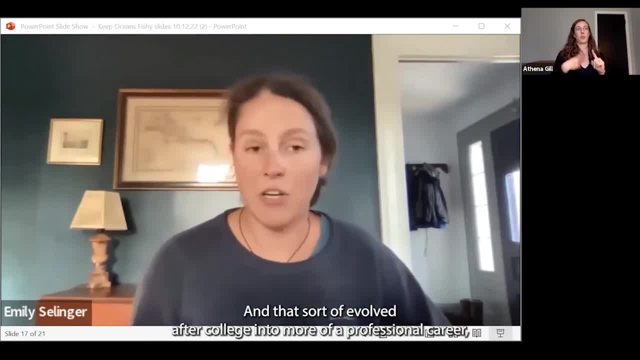 sailing as an early career And that sort of evolved after college into more of a professional career, working on schooners and sailboats as a deckhand, as an officer, as a relief captain up and down the coast, And that was really my, my first career. I, at a certain 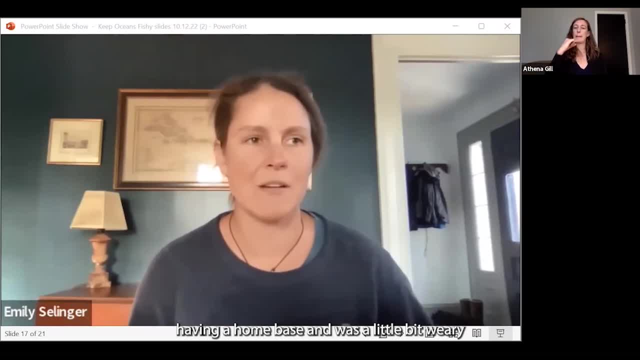 point, missed having a home base and was a little bit weary of the sort of nomadic lifestyle that comes with doing that kind of work. And I wound up back in Maine and, kind of just by chance, was introduced to aquaculture through a friend and very 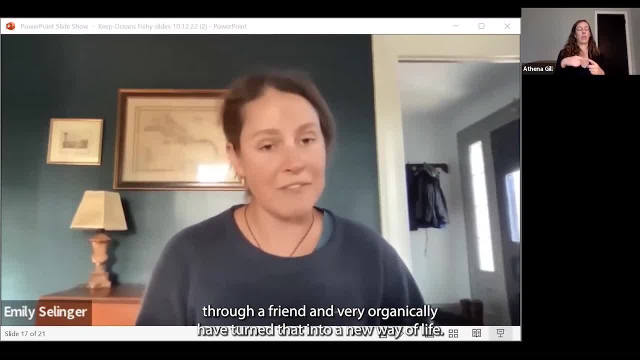 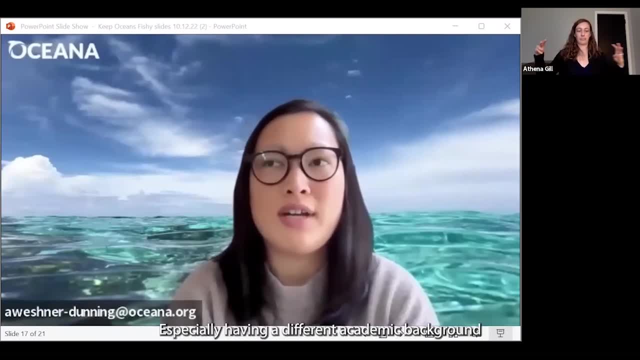 organically have turned that into a new way of life. Cool to hear that Just all of your lived experiences got you to where you are today, especially having a different academic background and then still being able to be in the marine science field. What 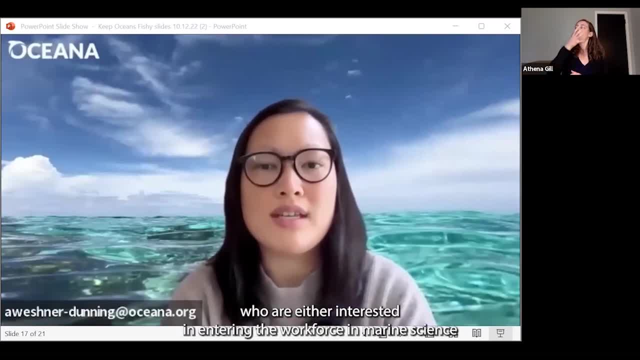 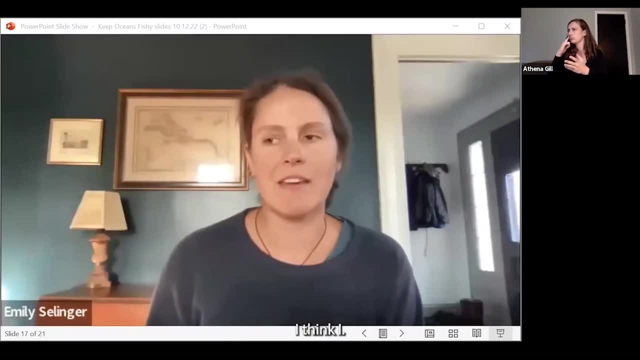 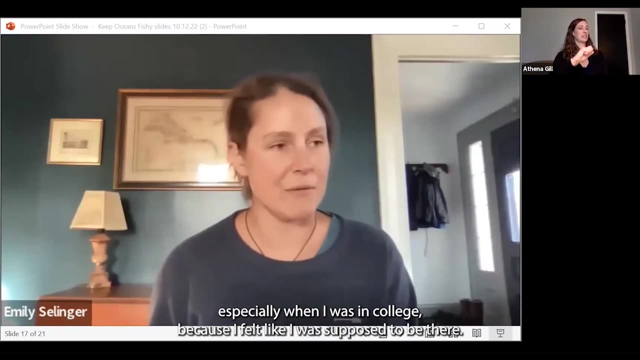 would be some advice you would give to young women who are either interested in entering the workforce in marine science or getting an academic background in marine environmental science. Um, I think I have really. I resisted this for a long time, especially when I was in college, because I felt like I 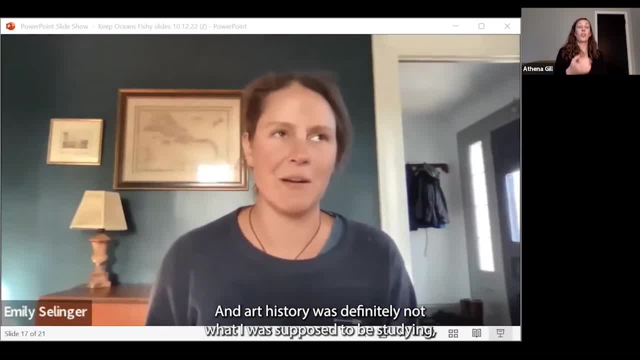 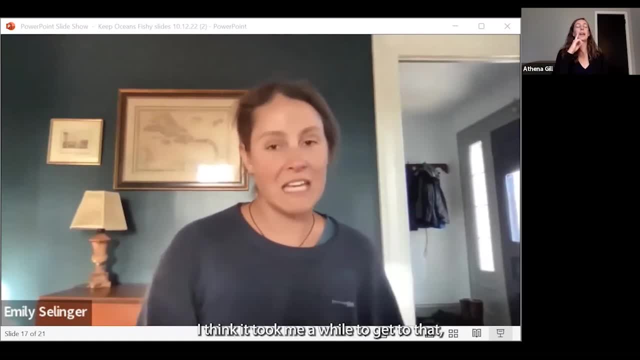 was, you know, supposed to be there, And art history was definitely not what I was supposed to be studying, but I wasn't sure what I was supposed to be studying at the time. I think it took me a while to get to that which was. 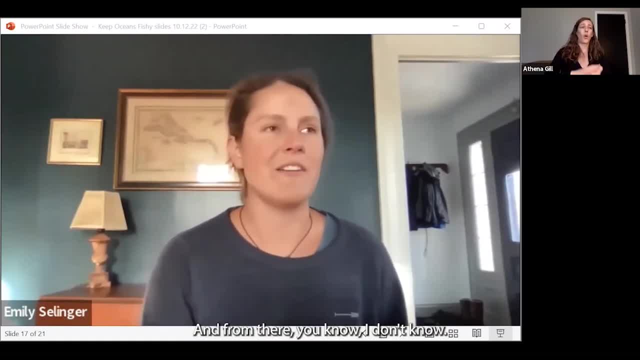 you know that I really just wanted to be on the water And from there, you know, I don't know- I just at some point I stopped worrying about it And I started to sort of be like Hey, like I want to be in Maine And like here's the thing I can do. 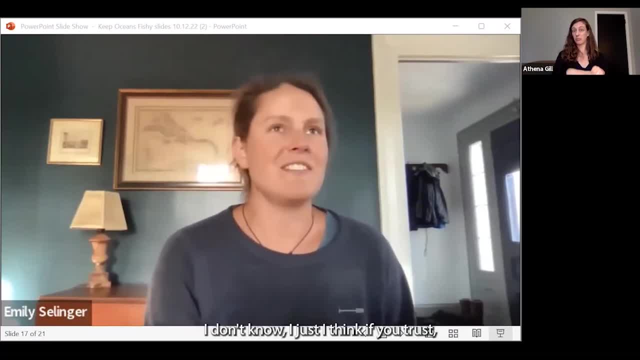 And I have all these skills And it seems fun And I don't know. I just, I just I just realized, knowing what you want to do, that if you want to do it, you generally will find a way to do it, And I 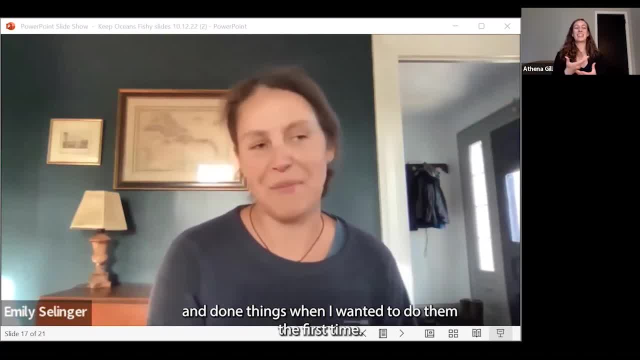 just wish that, yeah, I had worried less and done things when I wanted to do them the first time, I think, rather than kind of like dithering or like waiting or, you know, taking lesser jobs or whatever. I think, Yeah, we have a if we trust. 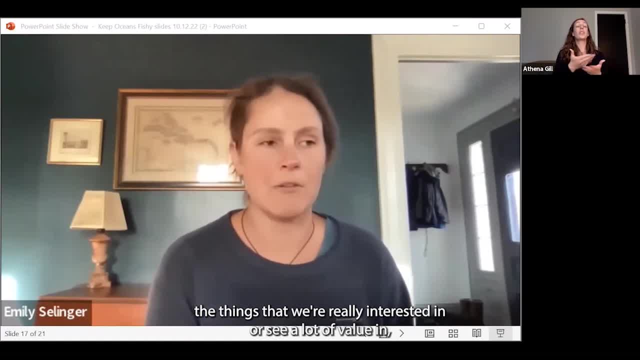 more when it comes to doing the things that we're really interested in or see a lot of value in, that thinks of a way of working out, or we find the ways to make them work out for ourselves. So yeah, yeah, no, I'm really glad you touched on that, Because I think 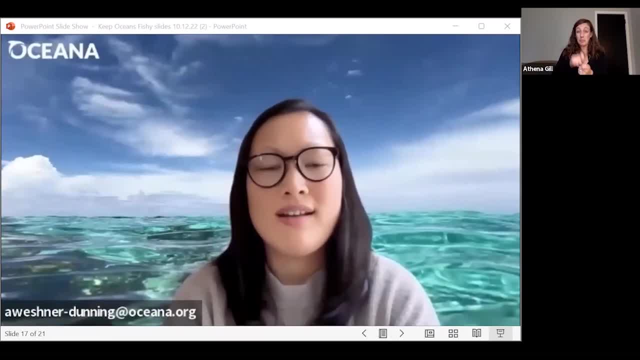 it'll resonate with a lot of the students, especially here watching tonight, that feel like they have to go into this academic background and marine science and there are other opportunities to be involved, Like if you find an interest that you like their way to get. 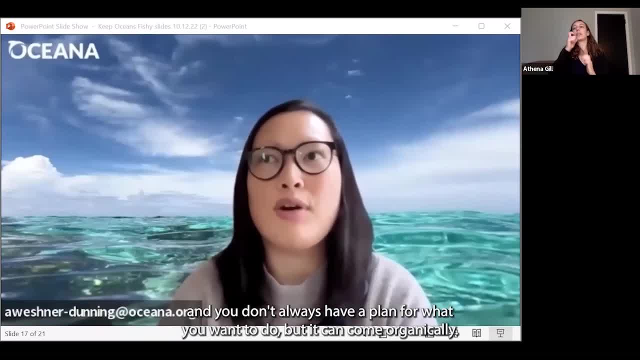 experiences, without necessarily always having to be academic and you don't always have a plan for what you want to do. But it can come organically And I think a lot of us have that same experience, And so it's really nice to hear someone who's a 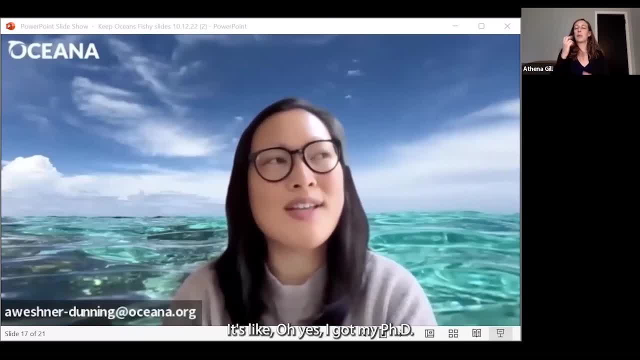 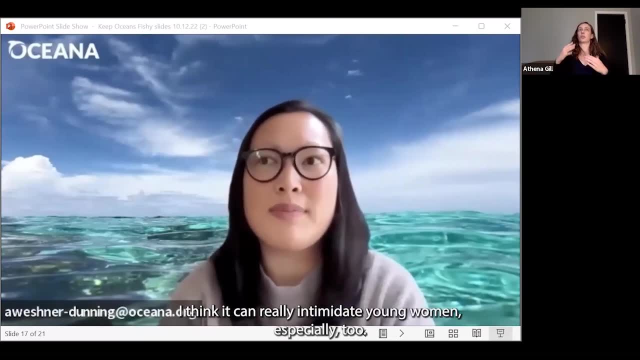 professional. share that, because I don't think a lot of people talk about that. It's usually like: Oh yes, I got my PhD at this age And I knew exactly what I wanted to do. I think it can really intimidate young women especially too. 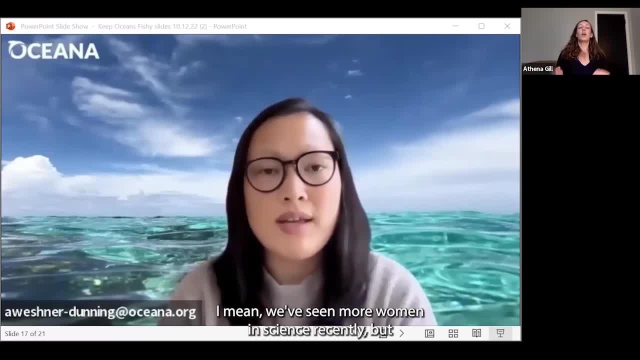 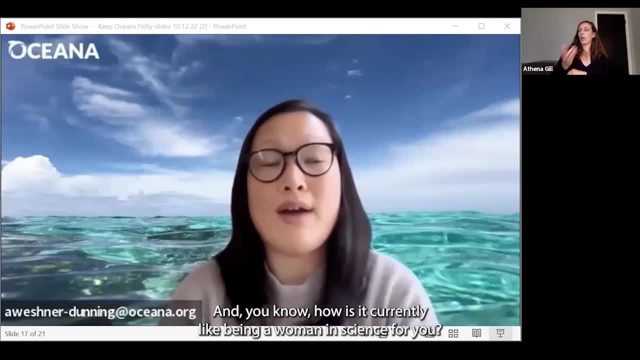 I mean, we've seen more women in science recently, but- and you know, you've really touched on being in an industry that's male dominated. So what was it like, And you know how is it currently like, being a woman in science for you. 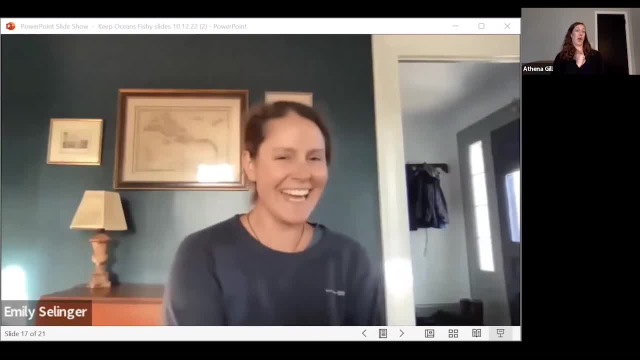 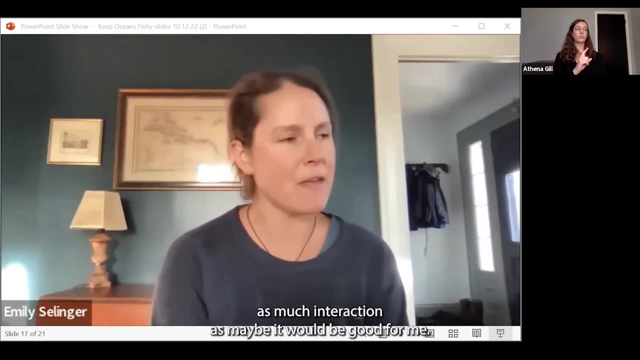 Well, it's great now that I'm my own boss And you know, I kind of like I'm in control of how much I interact with the industry, which you know because of my experiences I haven't, you know, I've been in this industry for a while now. 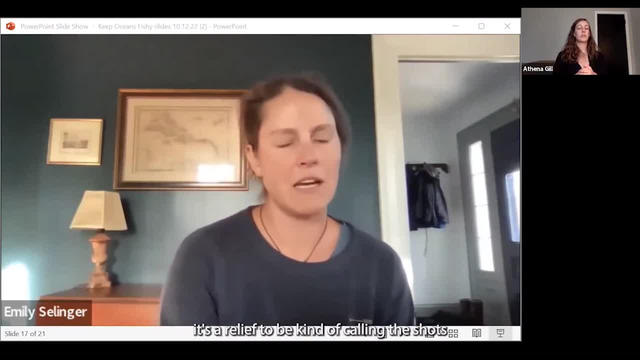 I've just been very focused and I've always thought that having a positive influence in the industry outside of science is maybe it would be good for me. But yeah, it's. it's a relief to be kind of calling the shots. Finally, I think for like. 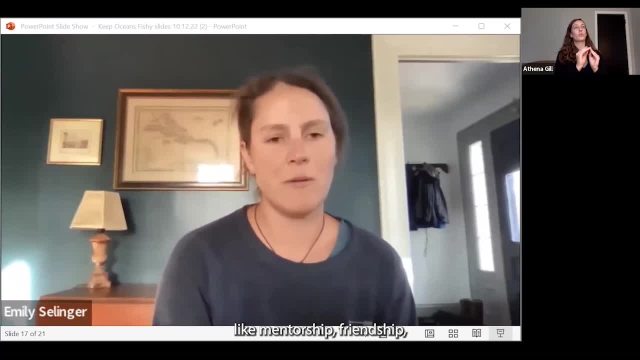 younger men, for women going in to male dominated and science related fields, like the thing I wish that I had done was seek out when they were there, which wasn't always, but I think that, like I don't know why it is, but we are so kind of on guard to defend ourselves, improve ourselves in those environments. 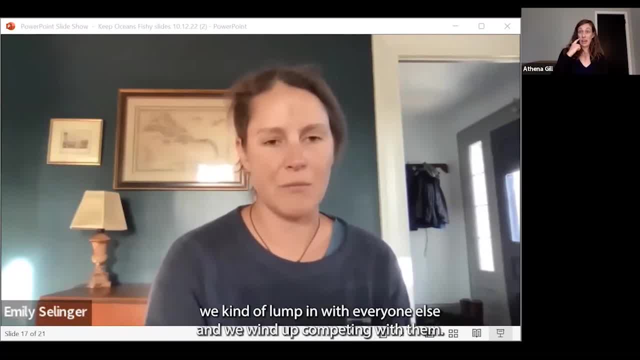 And that sometimes the other women around us, if they are there, we kind of lump in with everyone else and we wind up competing with them, and that, I think, helps none of us And I think, yeah, I wish that I had been more proactive about that and not just so. 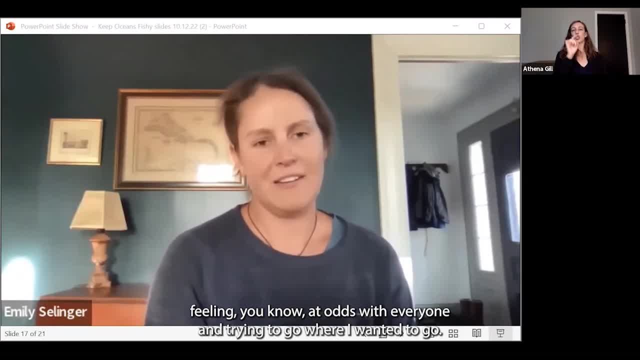 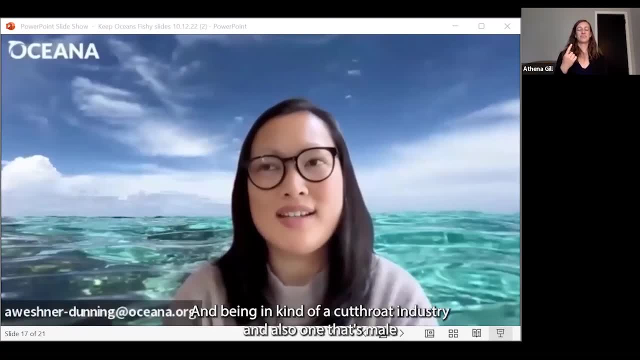 kind of feeling, you know, at odds with everyone and trying to get where I wanted to go. Yeah, yeah, I can. I can definitely relate to that as well and, being in kind of a cut throat industry and also one that's male dominated, it's hard to find your place and be heard. 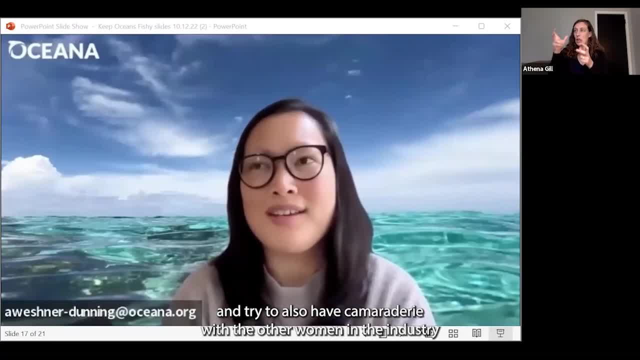 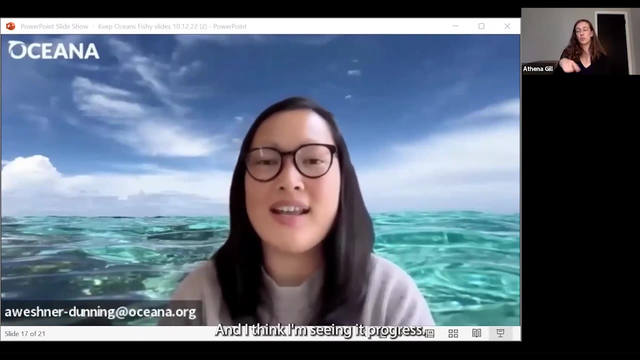 and respected and try to also have camaraderie with the other women in the industry, Without being too competitive, but also being strong and being seen, and it's just a very odd balance. I don't think it should be and it's sad that it has to be that way and I think I'm seeing. 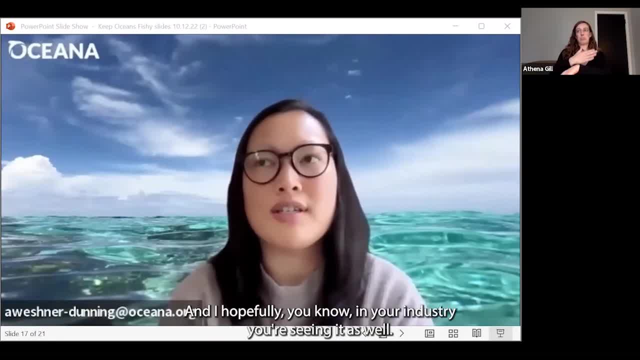 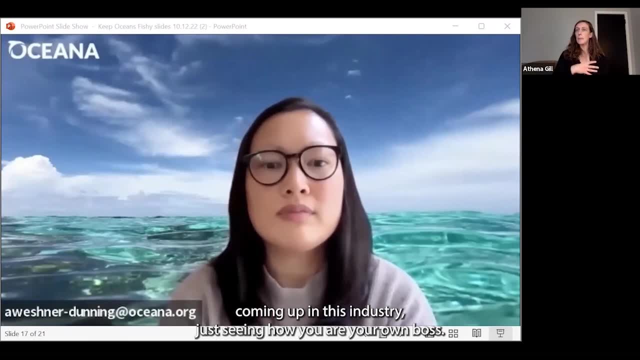 it progress And I hopefully you're. you know in your industry, you're seeing as well, but I think your story is definitely an inspiration to young women coming up in this industry, Just seeing how you are your own boss. they did it, you know, without you know. I had some. 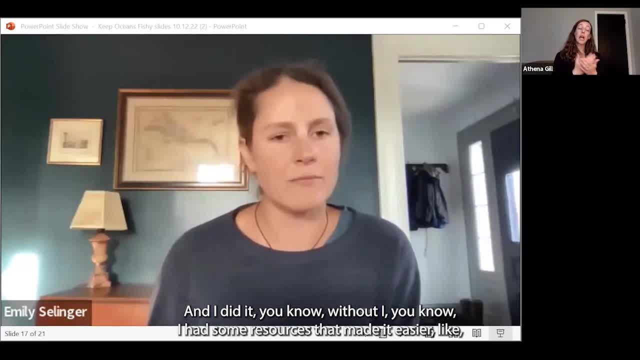 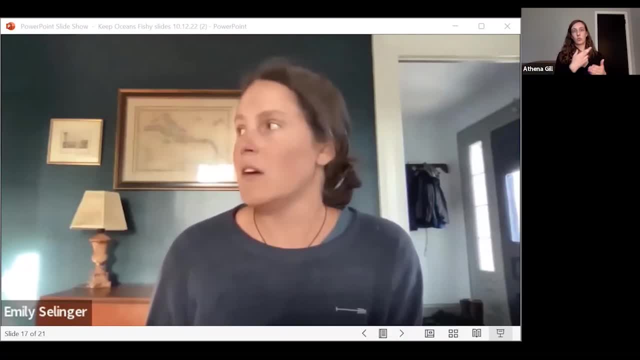 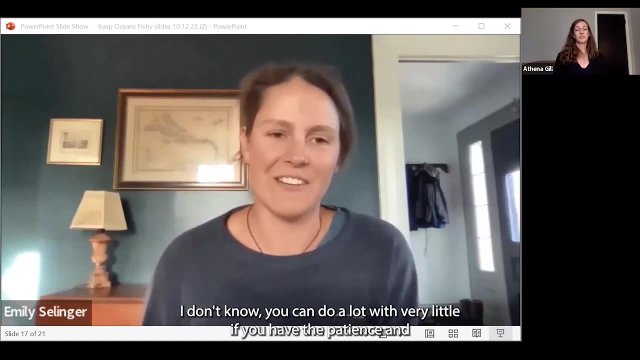 resources that made it easier. like you know, family history in the area and access to the waterfront that not everyone has and is definitely helpful, but I didn't really have a lot else. You know and it is I don't know. you can do a lot with very little. 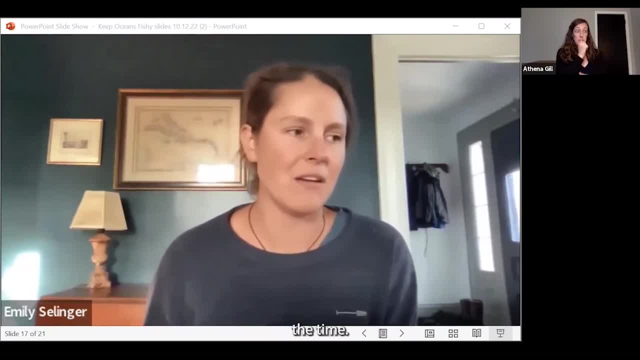 If you have the patience and the time- and I did make the effort to build some like really key relationships, with another woman Chiefly, who really like helped me out as I helped her out as we started. you know our own separate businesses nearby and, yeah, you can do a lot with not much. 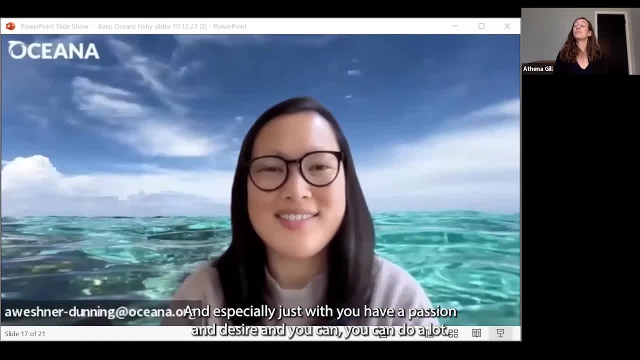 Yeah, and especially just with a passion and desire, and you can. you can do a lot. So, yeah, well, thank you for sharing. and then you know, Oceana is campaigning for healthy, abundant and sustainable fisheries policy. And so what does strong fisheries policy look like? 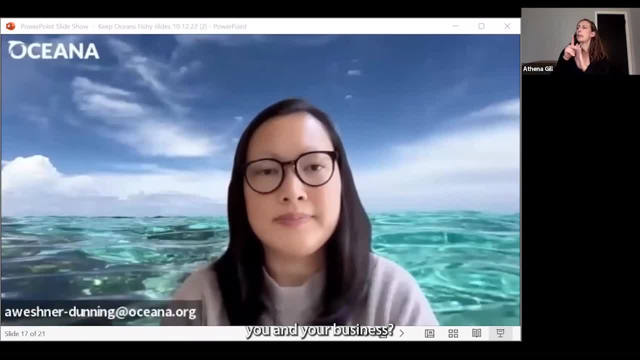 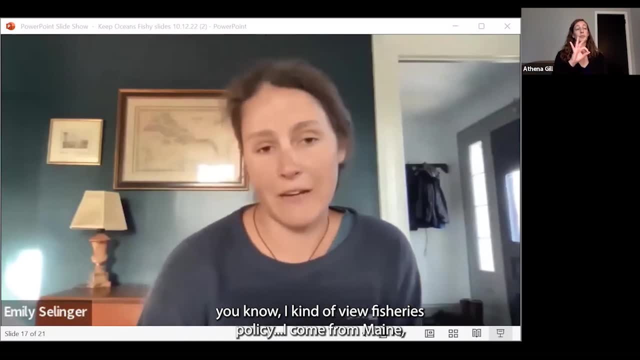 Yeah, What does that policy look like to you and your business? Um, I think that you know I kind of view fisheries policy. I come from Maine first of all, which is fisheries heavy place. our communities are very shaped independent by 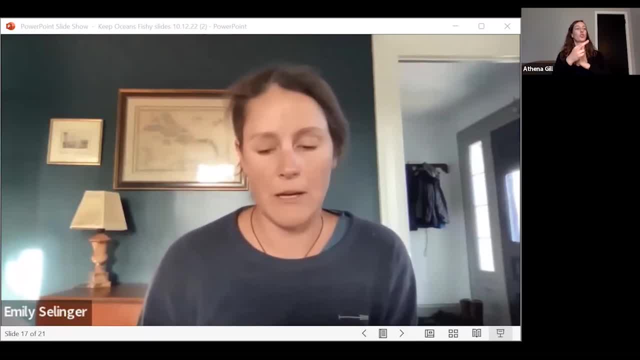 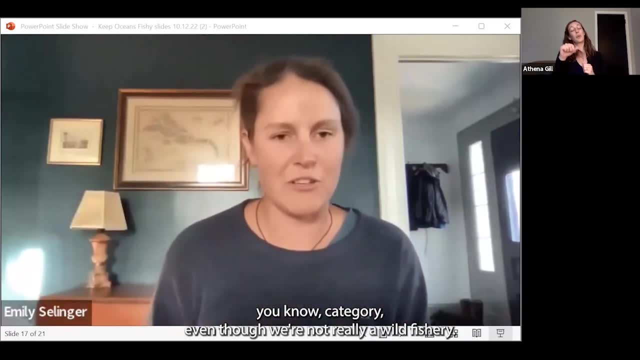 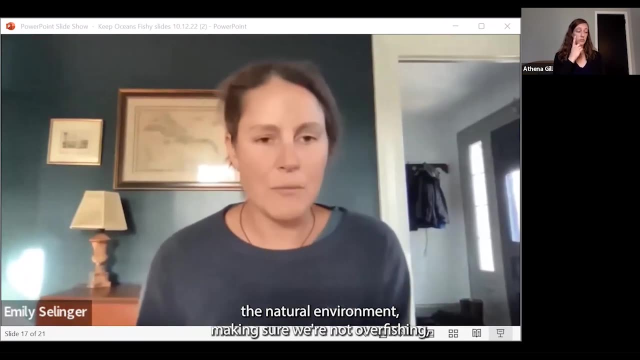 commercial fisheries, and more and more so by aquaculture as well, which kind of gets lumped into the fisheries you know category, even though we're not really a wild fishery. But I think everything from like protecting the natural environment, making sure we're 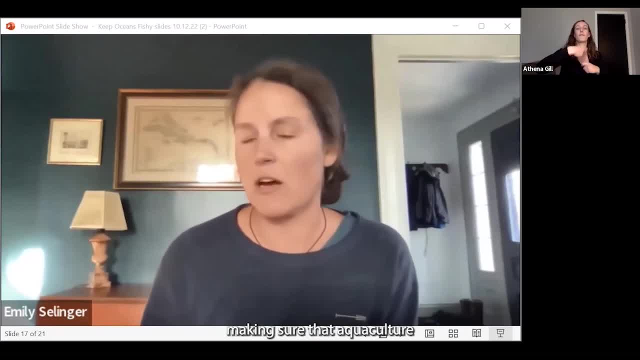 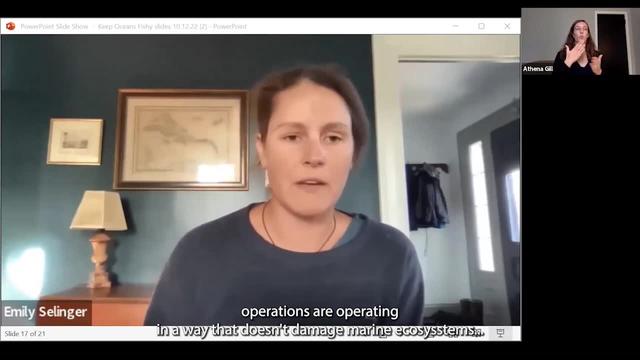 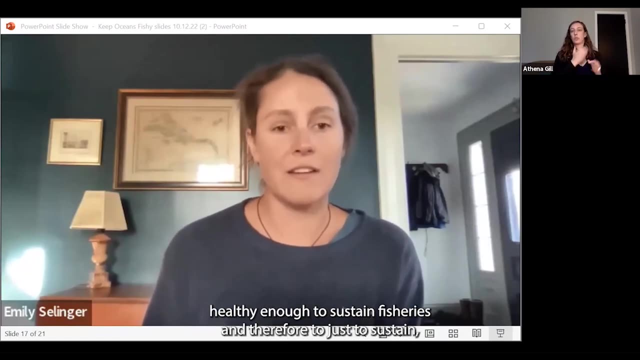 not over fishing, making sure that aquaculture operations are operating in a way that doesn't damage marine ecosystems. like all of that, is fisheries policy. that is essential to you know: keeping our oceans healthy enough to sustain fisheries and therefore to sustain, you know, the community that I serve. 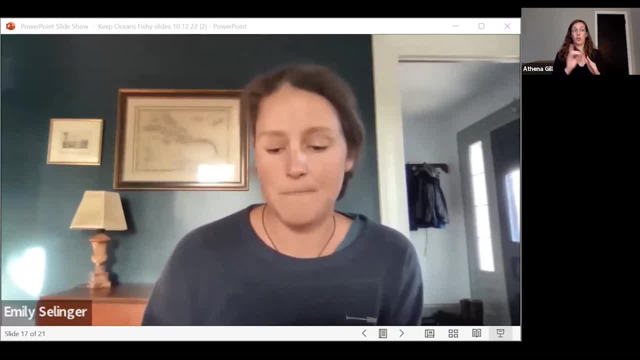 Yeah, And I think that's what I live in and my friends and my family And it's also in Maine. it's very baked into like our way of life and I think any manner you talk to, especially if they come from coastal areas, is like you know we have something. 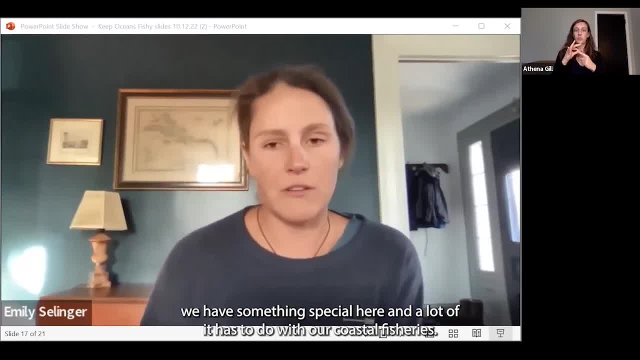 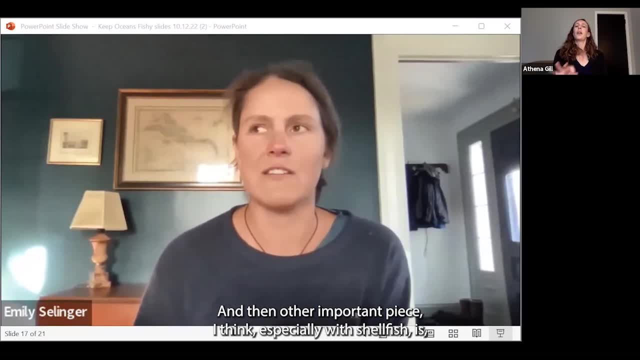 special here and a lot of it has to do with our coastal fisheries, so it's very much tied into that. And then the other important piece I think especially with shellfish, is, you know that good fisheries policy kind of translates Pretty directly into the public trust in our product and the quality of the product. 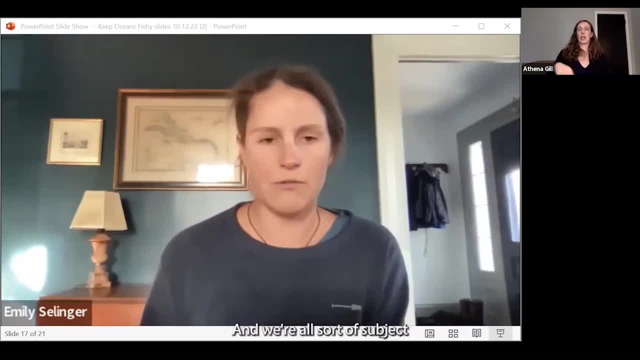 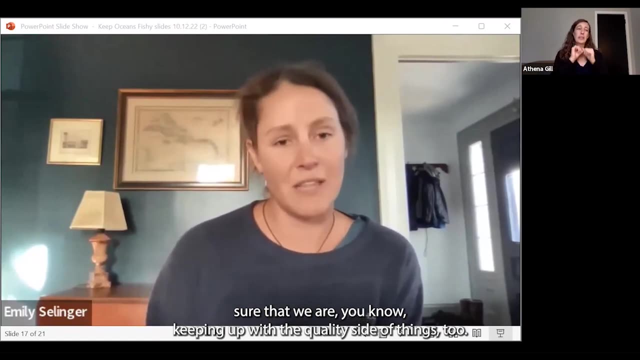 that goes to market And we're all sort of subject to the same kind of larger brand of Maine seafood- and for me, you know, oysters that come from Maine and good policy, just make sure that we are, you know, keeping up with the quality side of things too. I think that that is really. 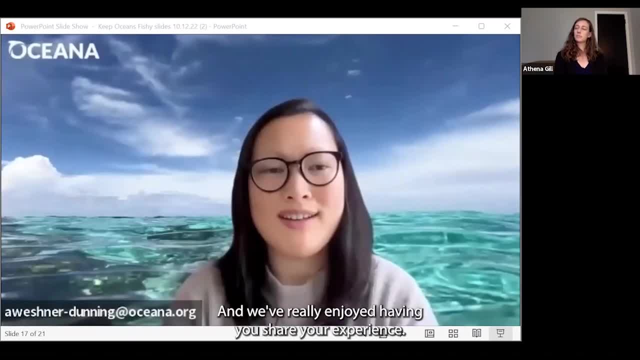 important as well. Well, thank you so much, And we really Enjoyed having you share your experience. and, yes, if anyone has any questions, we will be able to put up your contact information on our slide. Yeah, so All right. 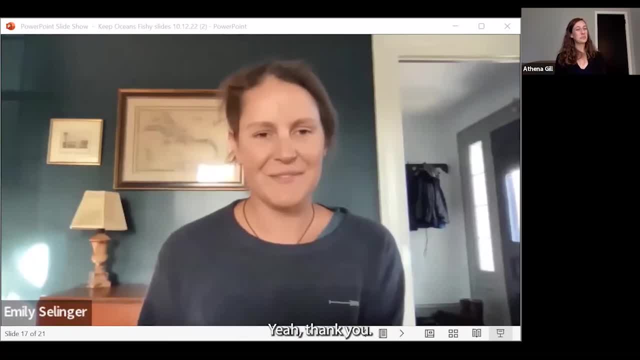 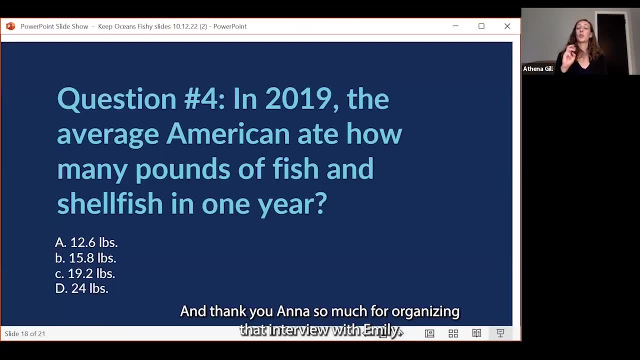 Thank you so much. Yeah, Thank you Hi. Okay, that was Emily of Emily's oysters, and thank you so much for organizing that interview with Emily. And now we've got our final poll. Okay, In 2019, the average American ate how many pounds of fish and shellfish in one year? 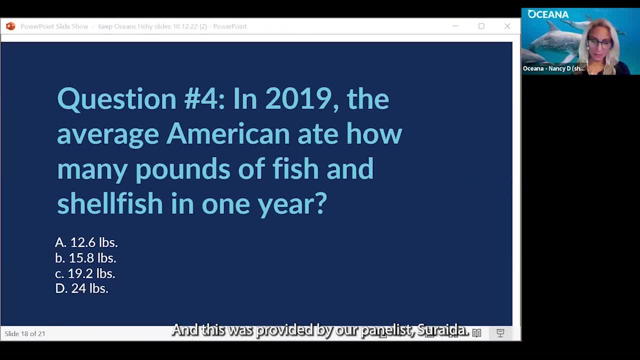 And this was provided by our panelists, Sarita. Thank you, Sarita, for that question. I know for me personally it would be like 1000 pounds. Oh, it's a tough one, folks. which ones are going to be? And actually, Sarah or Anna? I realized I've written the wrong answer on the bottom of. 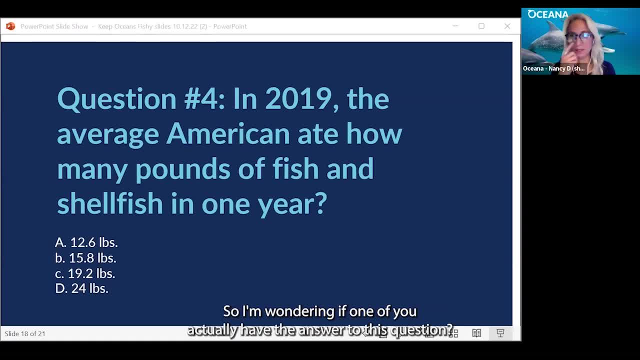 my poll question, so I'm wondering if one of you actually have the answer to this question. Yeah, the answer is see 19.2 pounds. so we had 18% of folks get the right answer on this one. that was based on 2019 statistics, which was a slight increase of point two pounds. from 2018.. I just for reference: the USDA dietary guidelines for Americans recommends That people eat to four ounce servings of seafood each week. this would be 26 pounds per year for an individual. Thank you, Sarah, All right. 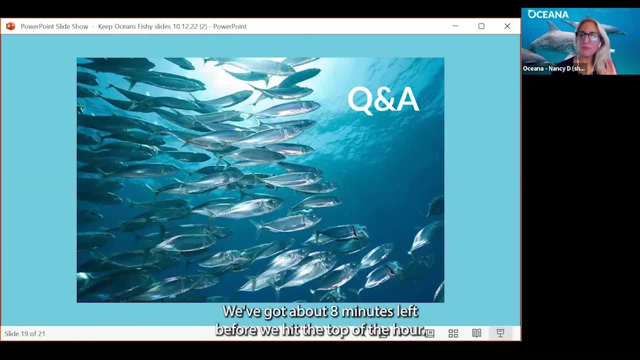 And now I'd like to open up the floor. we've got about eight minutes left before we hit the top of the hour and I think we may have a handful of questions for our panelists. And we had some great questions in the q amp a functionality, so if you do have others, you'd 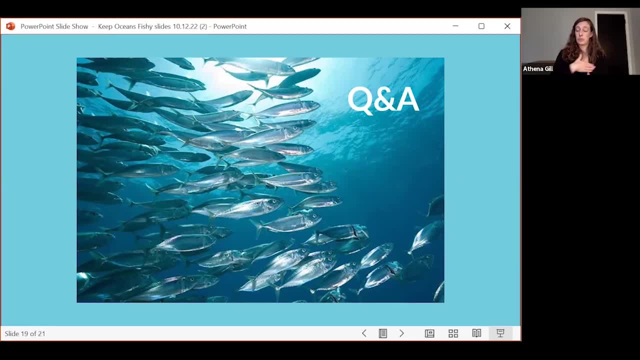 love to ask and encourage you to do so. I met one question that that a few of our panelists have answered but I thought it'd be great to put to the group is: why do you think that women are leading this effort versus men? Take that, Yeah, I can start off, because I answered that slightly in the chat. 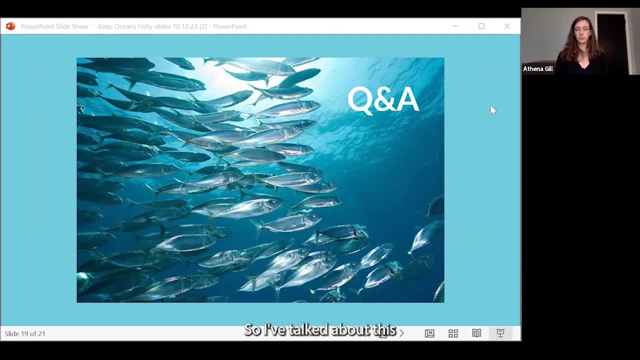 Um, so I've talked about this specifically because the groups I have worked with recently have been all women, were, as my education and past and other fields were predominantly men focused or lead, And so we kind of just as we're like out in the field together like, oh, we're all women. 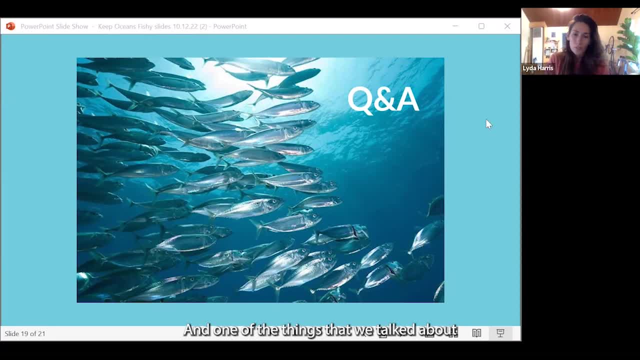 like why, And one of the things that we talked about was that women are traditionally the ones that carry a lot of the emotional burden for communities as well as are the traditional caregivers for the family or community unit, And so that often translates to caring about the earth as an extended family member or 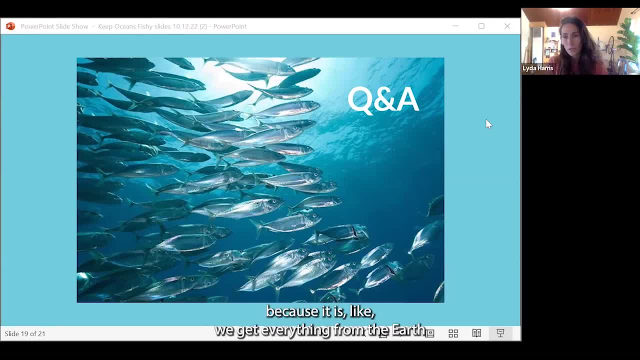 an extended Unit of the community because it is like we get everything from there And thinking about the children and the grandchildren and will they have food and resources moving forward? And so when you look at who's currently leading a lot of- especially the youth, environmental 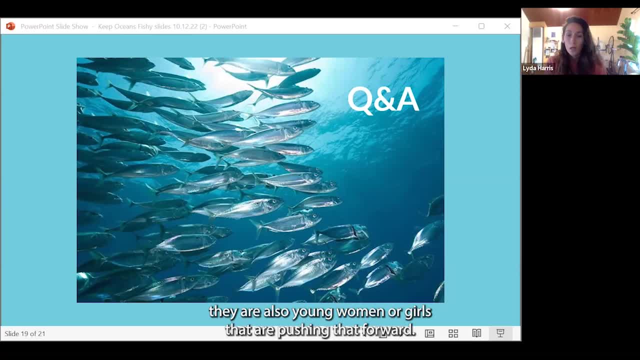 movements. they are also young women or girls that are pushing that forward, and so we see that time and time again. Um, it's not necessarily a bad thing- I love being in that space- but it is definitely a space where it's predominantly women often, and that can have other systemic impacts and effects, especially when 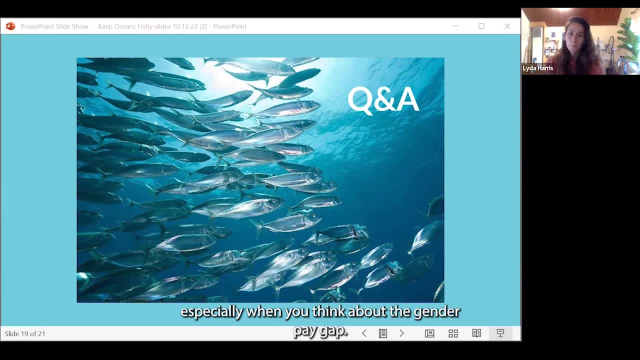 you think about the gender pay gap? Okay, Okay, do we have any other questions for the panelists? I'd love one of you just maybe highlight this idea of not being afraid to seek out a mentor. like as you are, early stepping out the door can be a little scary: getting started in ocean conservation and fisheries, knowing where to go, and was there someone who maybe 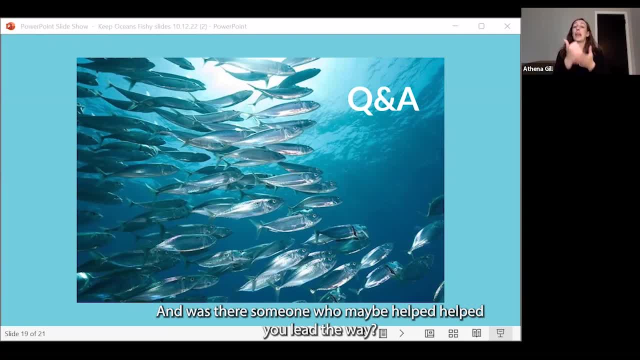 helped, helped you lead the way? Um, we can answer that one. so we focused a lot on mentorship. So, especially- I think you brought it up- is it lighter than I current that about? you know, there are a lot of women now, more even in Noah, so we just had our, you know, the report. 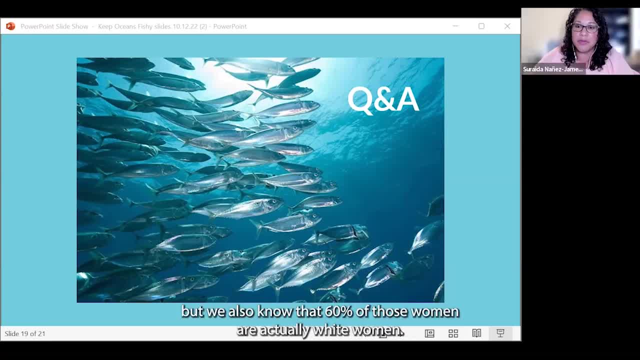 But we also know that 60% of those women are actually white women. so having mentorship In the beginning, You know it, when I did marine fisheries, There was no women at the college that I would teach you in classes like not even one. 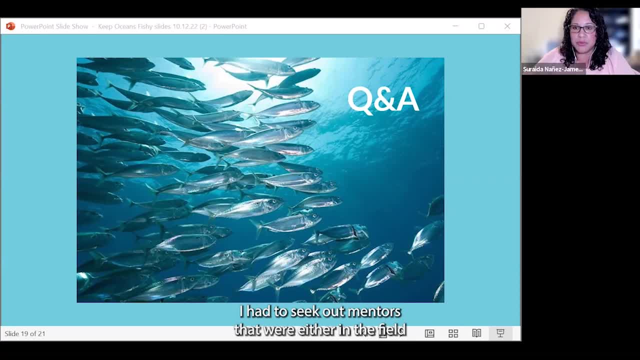 And so when I had to seek out mentors that were either in the field or going into the field or just that have representation- The biggest one, I think, that really influenced me. she was in my graduate school, so she was actually the Dean for science and engineering, and she- she has an amazing background. 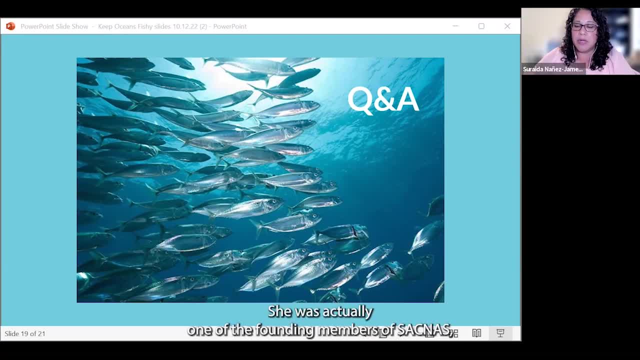 She was actually the Dean for science and engineering and she, she has an amazing background. She was actually one of the founding members of sadness, which is a society for the investment of Chicanos and Native Americans in science, and has been my mentor to this day. 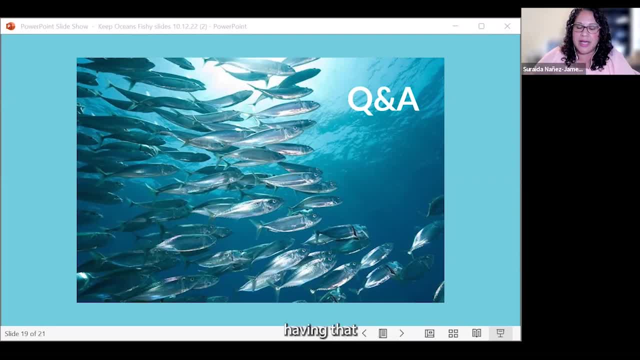 But I think you having that, that perspective of somebody who's been in the field, who's gone through some of the things that maybe you will or not go through- because I know I went through a lot of different things, being, you know, a woman and then also 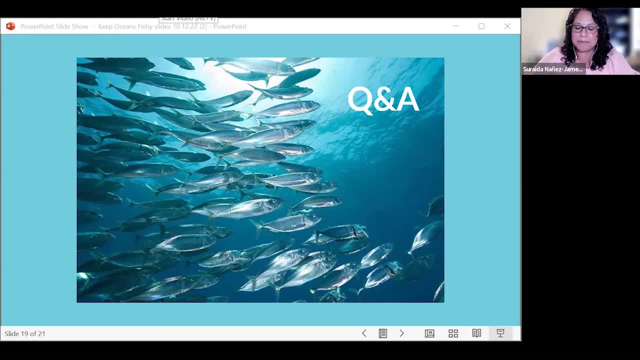 being a minority. so another layer to that being a minority, so another layer to that being a minority, so another layer to that. I think it helps. you have to build a community. I don't think you can't do it alone. I would say everything I've done, I've done because somebody has helped me along the way. 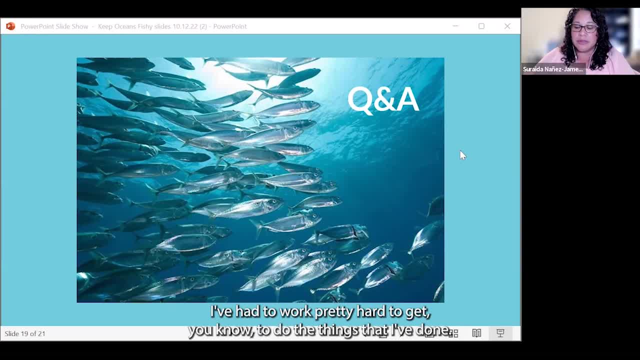